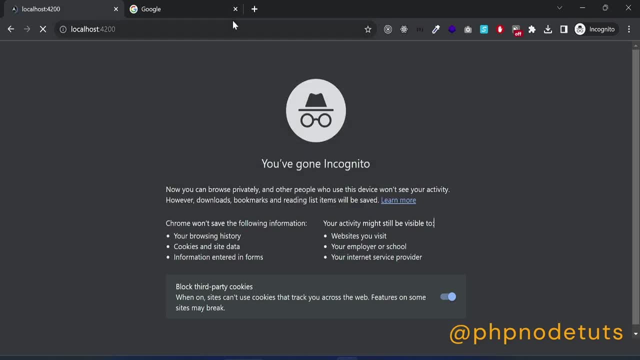 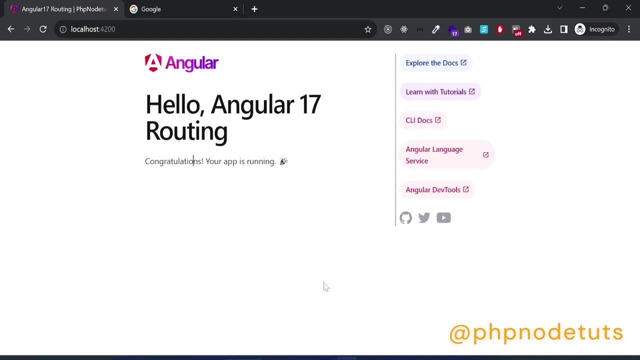 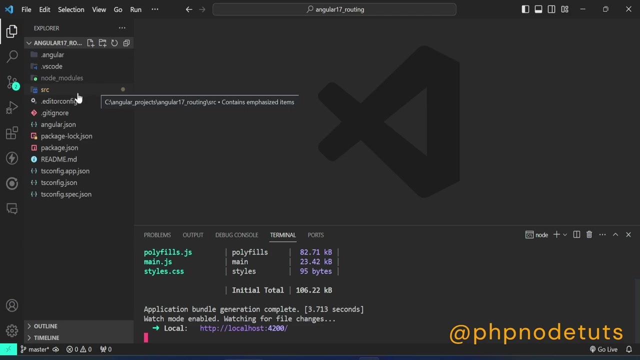 Now open your browser and type localhost colon 4200 and you can see the Angular 17 page with new Angular logo. Now let's see the directory structure of Angular 17.. The src folder is the main folder. The app folder contains the components, templates and styles for your 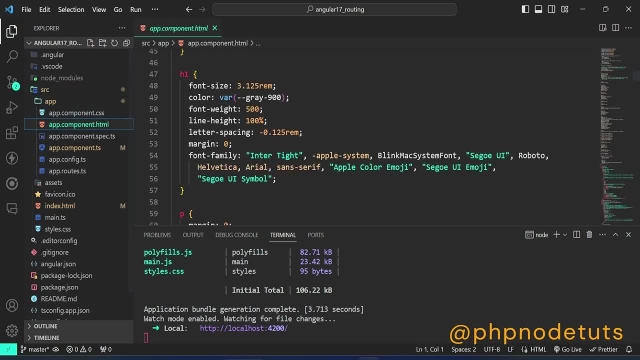 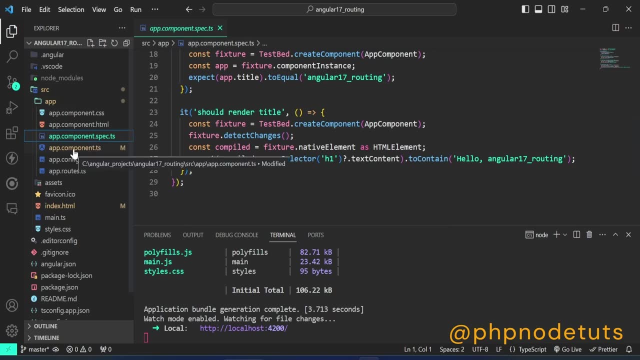 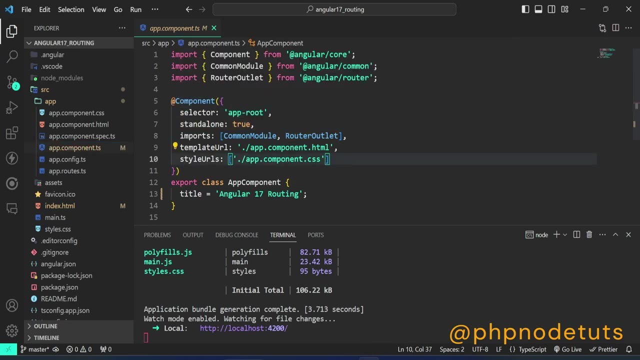 application. This is the CSS file for app component. This is the HTML file for app component. Test file for app component. This is the TypeScript file for app component. You can see that this component is a standalone component. Router outlet is imported and added inside imports array. 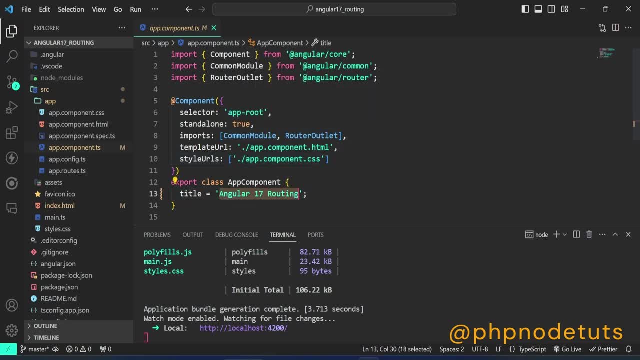 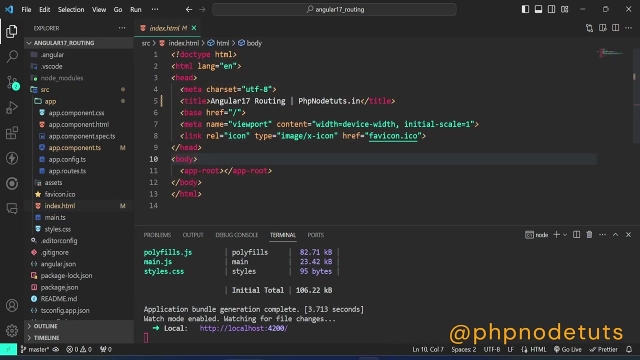 Add title for app component. This is app config TypeScript file. This is the approotts file. We will add the roots inside this file. This is indexhtml file. You can see app root selector where the content of the root component will be rendered in the HTML file. This is maints file, which is the main entry. 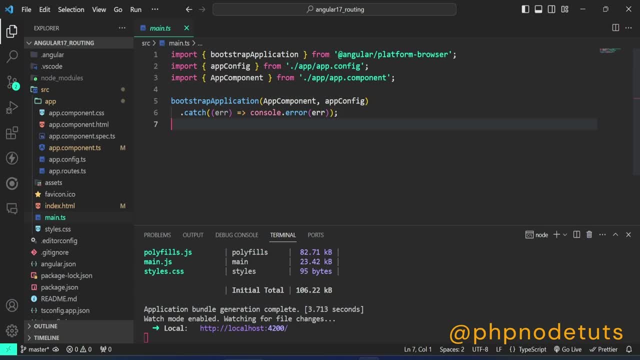 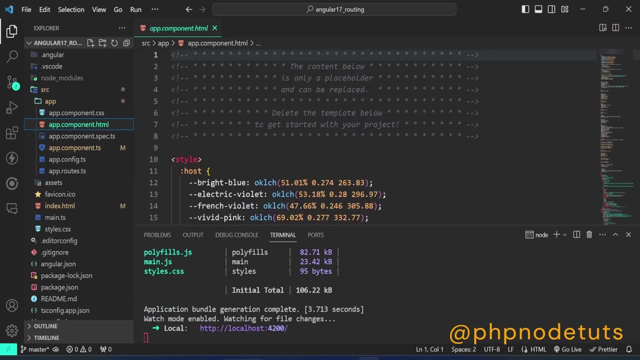 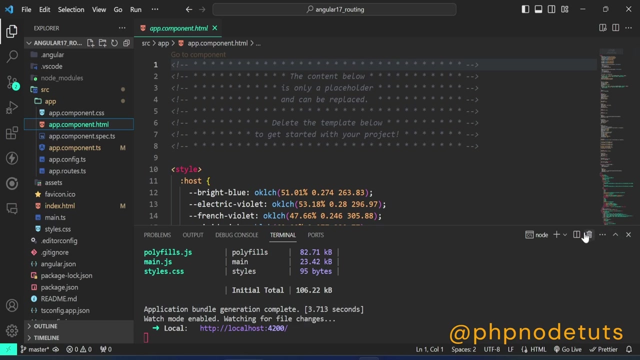 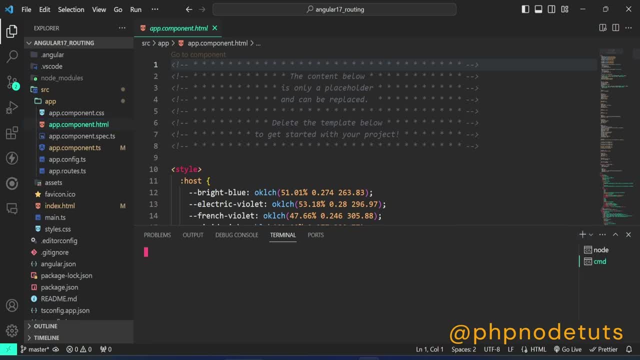 Click on this icon and select command prompt to open a new command prompt. Now type the command ng: generate component home dash dash. skip dash tests. This command will create homecomponentcss, componenthtml and homecomponentts files inside app slash home folder. 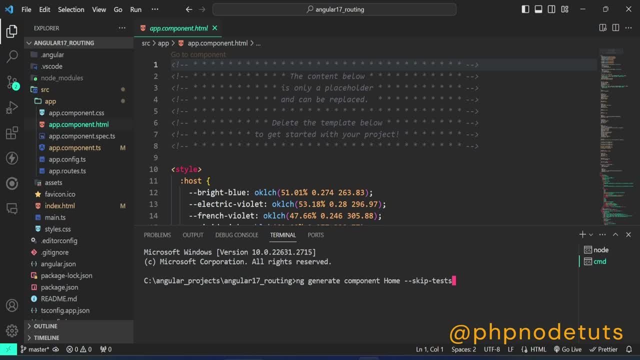 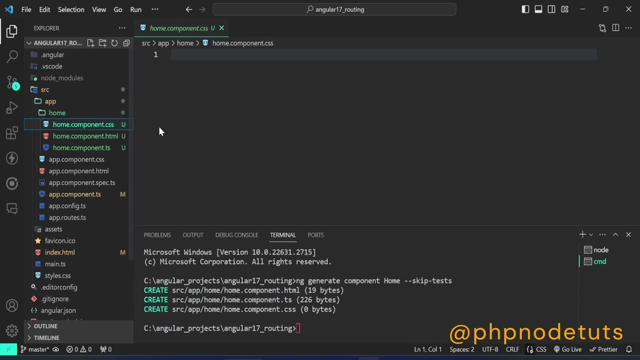 It will not create spects test file. You can see that home folder is created and homecomponentcss, homecomponenthtml and homecomponentts files are created in the home folder. Now type the command ng: space g, space c, space about space. dash dash, skip dash tests. 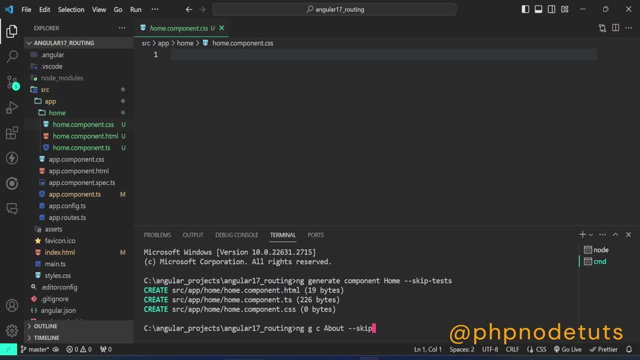 Here g is for generate and c is for component. This command will create aboutcomponentcss, aboutcomponenthtml and aboutcomponentts files inside app. slash about folder. It will not create spects test file. You can see that about folder is created and css. 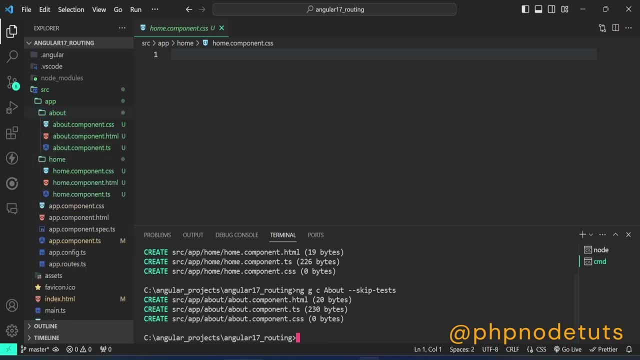 html and ts files are created in the about folder. Now type the command ng space g, space c, space, contact space. dash dash, skip dash tests. This command will create contactcomponentcss, contactcomponenthtml and contactcomponentts files inside app slash contact folder. 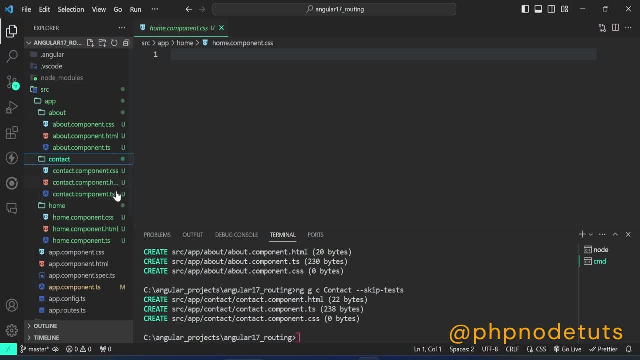 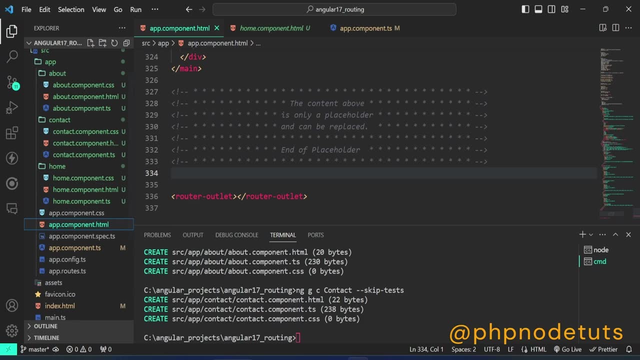 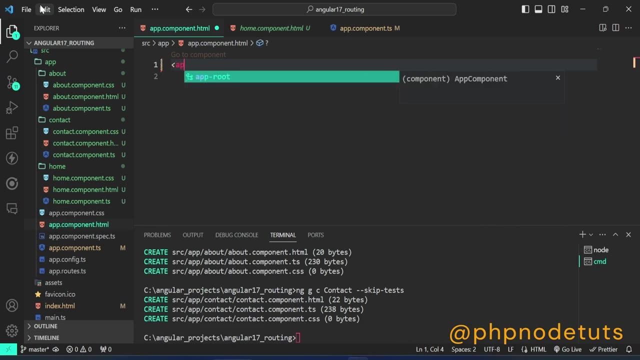 It will not create spects test file. This command will create contactcomponentcss file and contactcomponentts files inside app. slash contact folder. Open appcomponenthtml file and delete all the default html Here. add app home selector, which will be used to display home component. 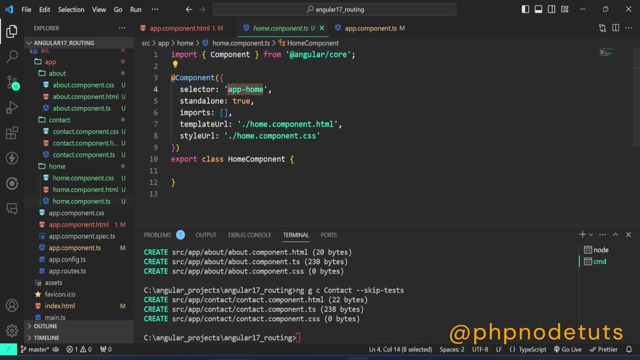 Open homecomponentts file. You can see that the selector name is app-home. Open aboutcomponenttms ts file. Here the selector name is app-about. Here the selector name is app-contact. Now, after app-home selector, add app-about selector and app-contact selector. 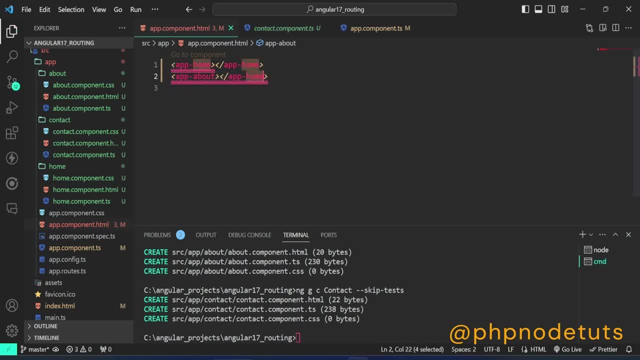 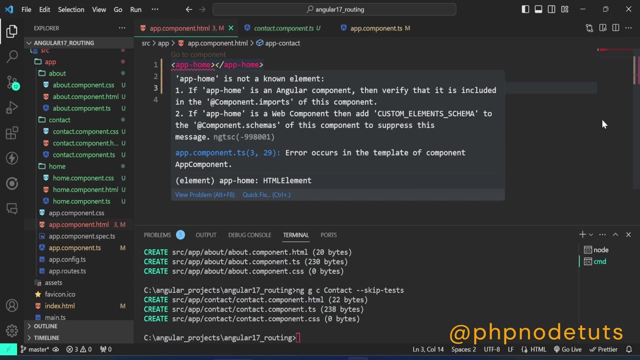 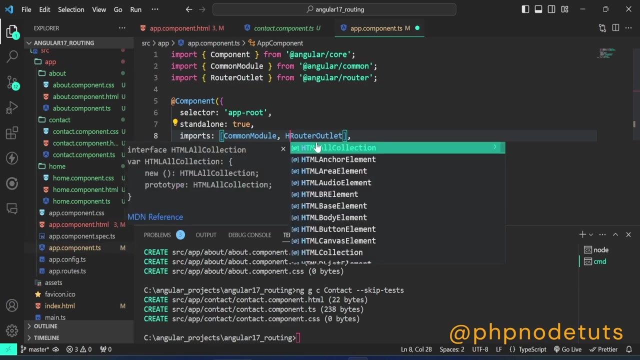 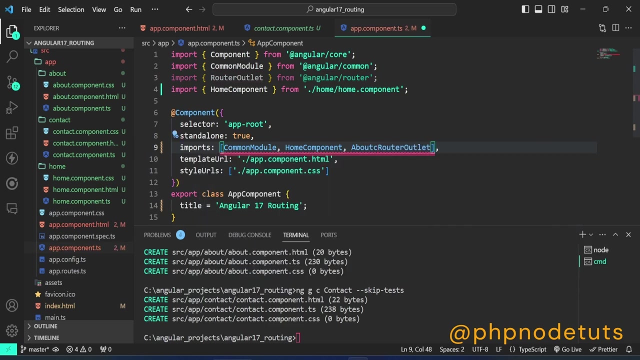 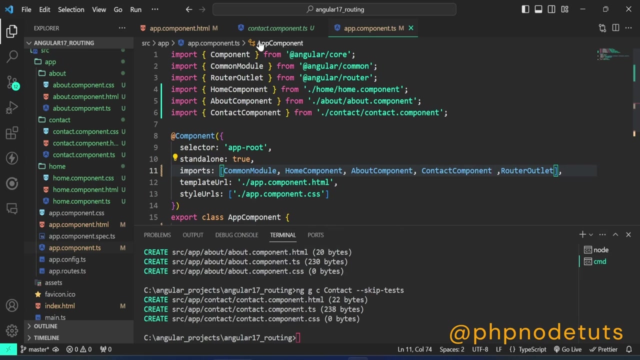 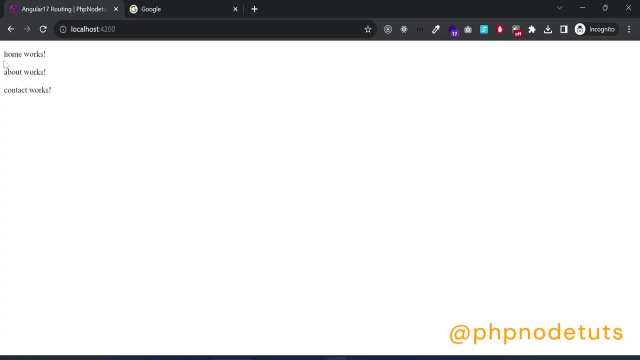 Here you can see: app-home is not a known element error. To fix this: open appcomponentts file and import home about and contact components and add them in the imports array. Now you can see that the error is gone. Now open your browser and you will see that all the components 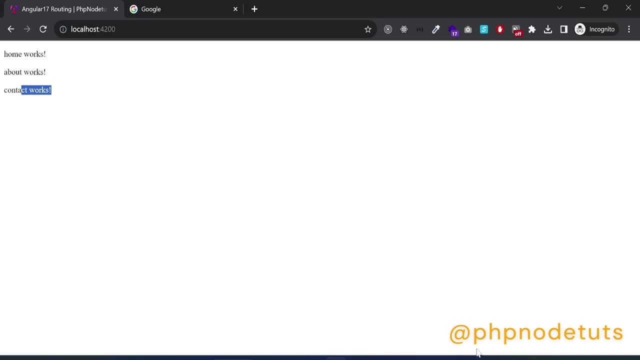 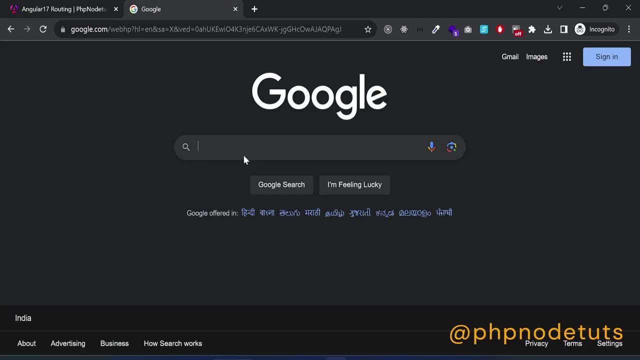 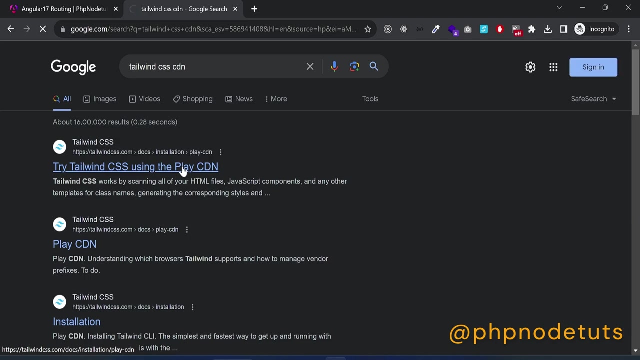 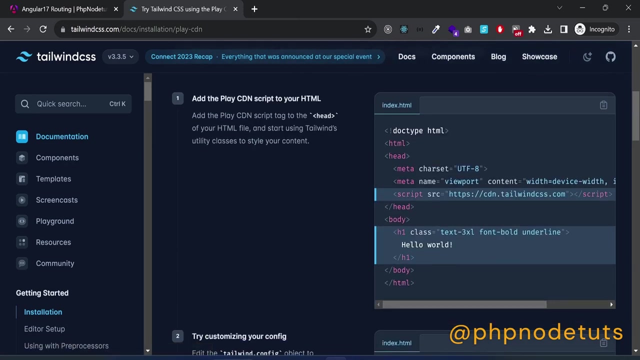 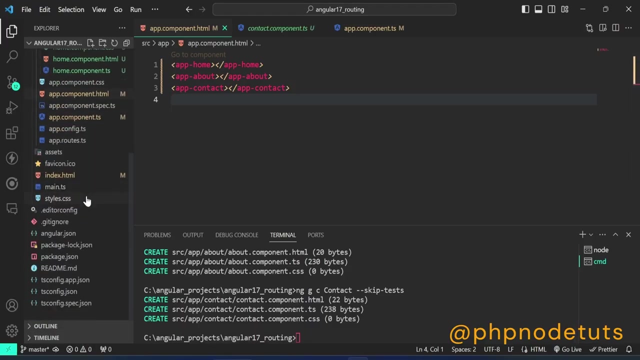 have been rendered. Now let's add Tailwind CSS CDN in our app for styling. Open googlecom and type Tailwind CSS CDN. press enter. Open this link. Copy the script tag. Open indexhtml file. Paste the script tag here. 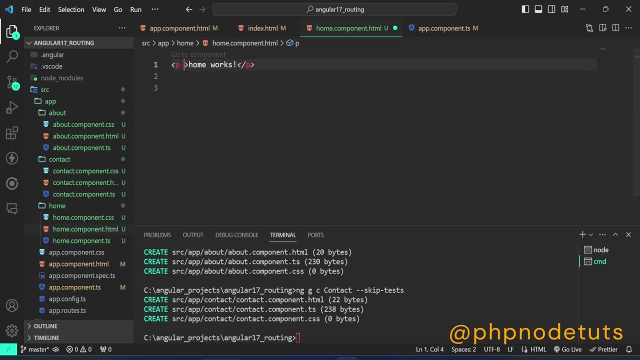 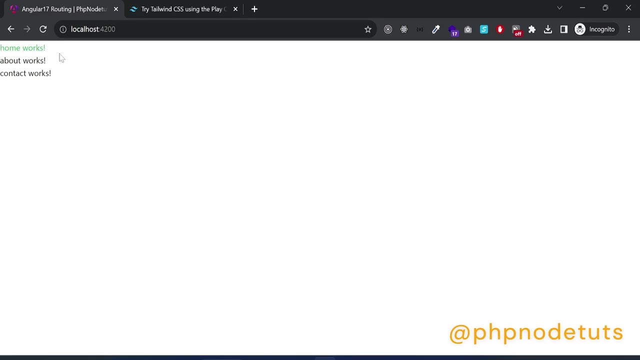 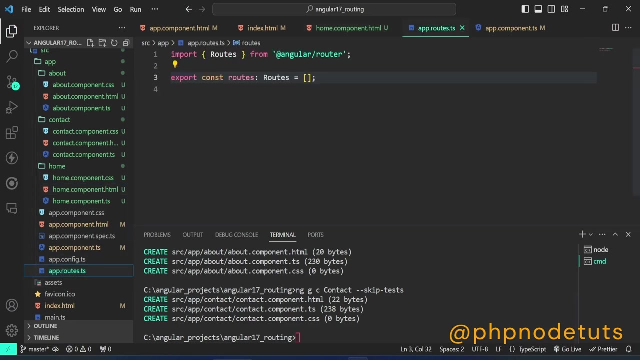 Now let's add Tailwind CSS classes to check if the CDN is working or not. Now open your browser and you will see that Tailwind CSS classes are working. All the fathers have been applied to the text. Now open approutests file to add the roots. 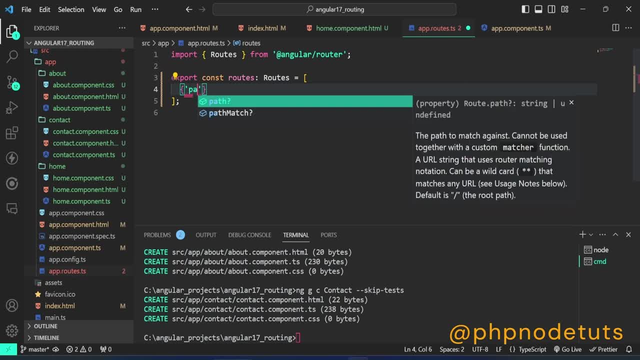 In curly braces type path in single quotes followed by a colon and a single quote. then add a comma. Include component followed by a colon and the home component. Don't forget to import home component. Add a comma after the ending curly brace. 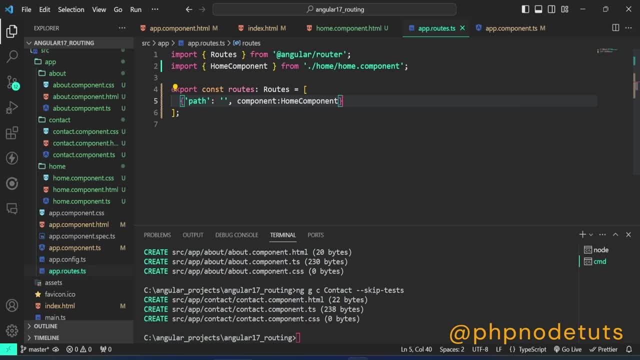 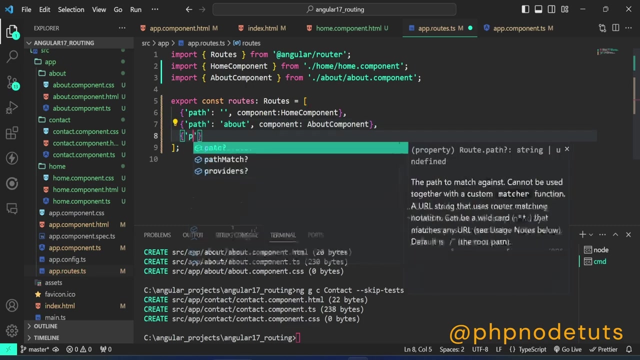 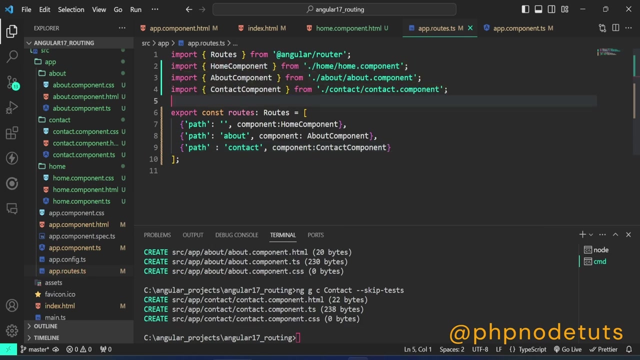 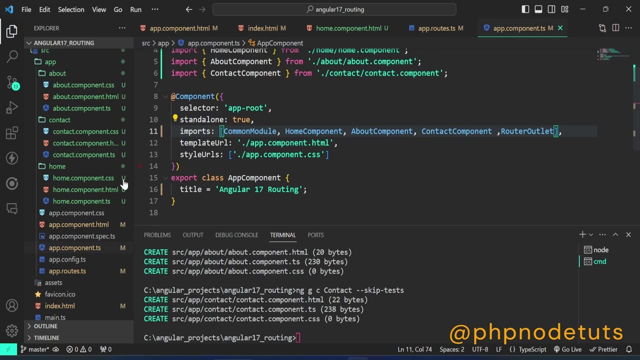 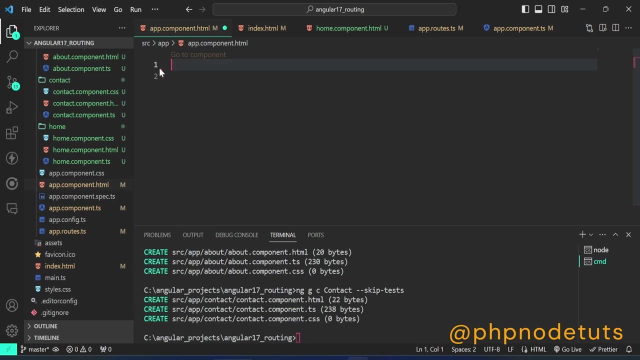 After the home root, now add a root for about: Import, about component: Now let's add contact root: Import contact component. Open appcomponenthtml file and remove all the selectors. Now add router outlet directive, which acts as a placeholder that Angular dynamically fills based on the current router state. 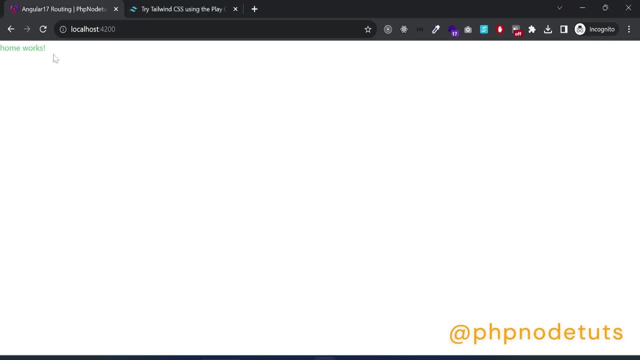 Now open your browser and you will see that only the content of the home component is displayed, as this is our home root Now. type localhost colon 4200- slash- about to open the about root. Now type localhost colon 4200- slash- contact- to open the contact root. 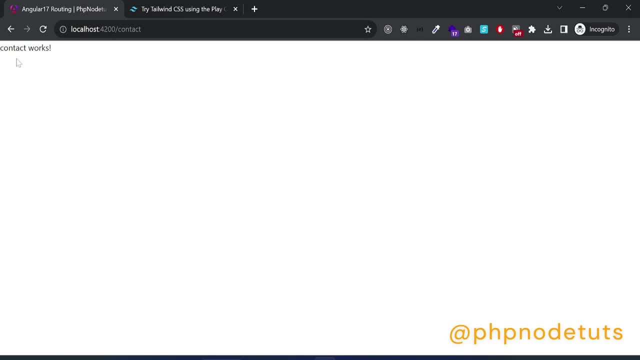 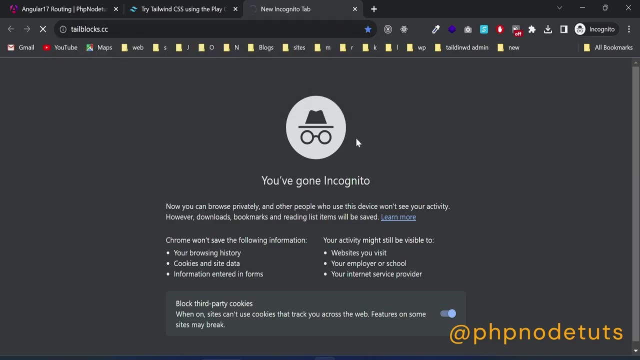 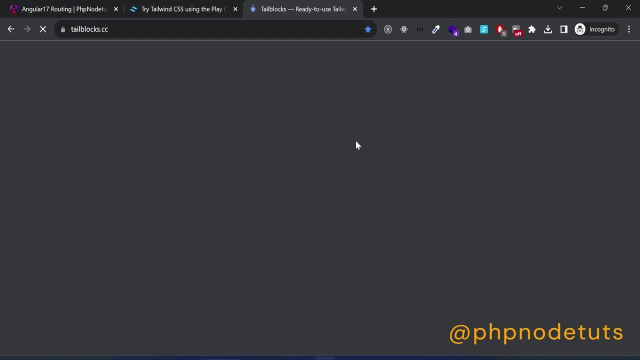 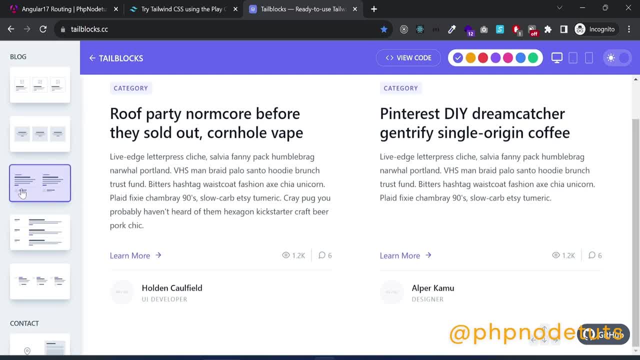 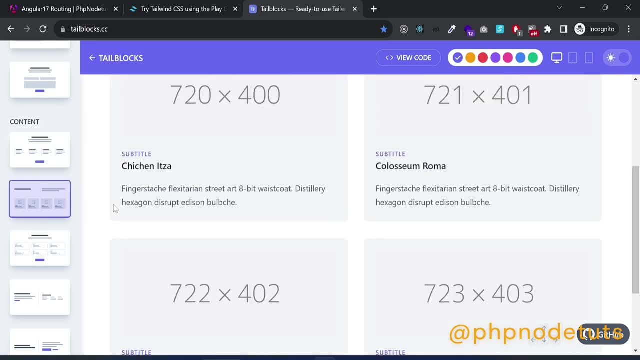 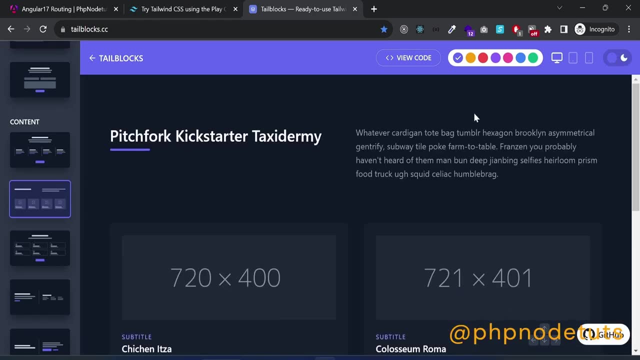 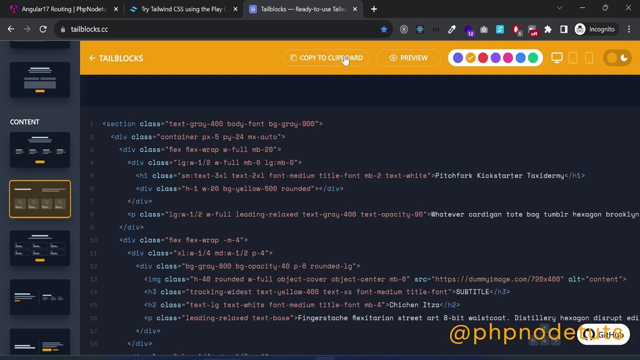 Scroll down, Select this template block and click on dark mode icon. Now click on yellow color. Now click on view code and copy the code. Now we will add template for about component. Scroll down: Now we will add template for about component. 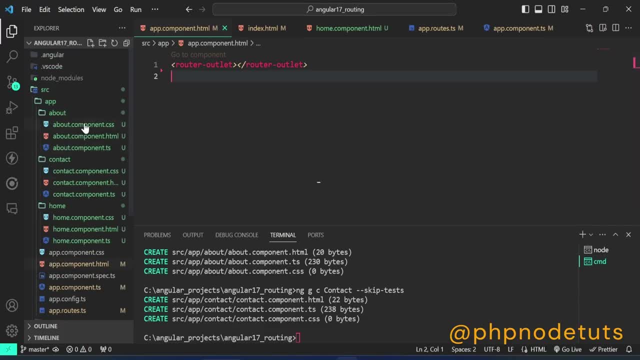 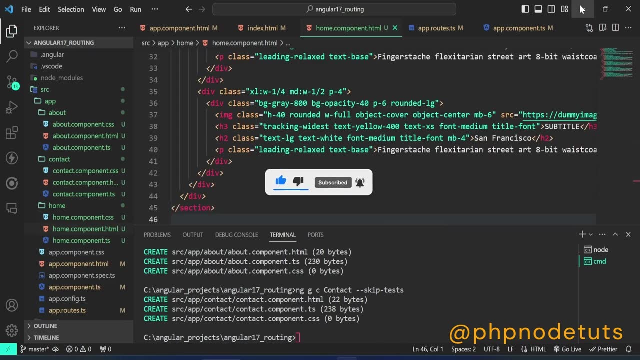 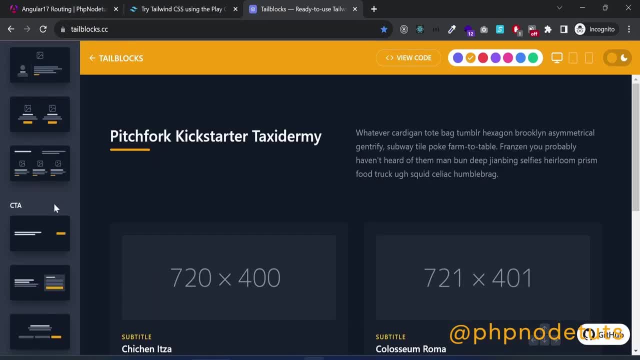 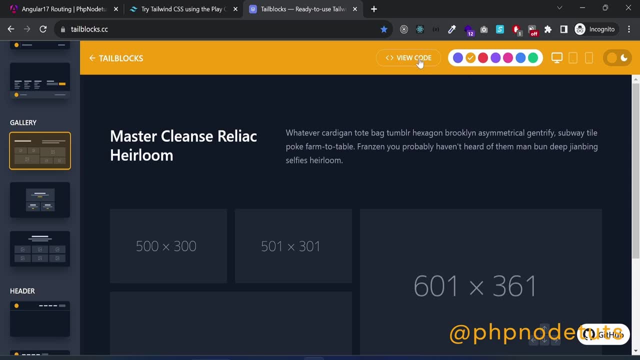 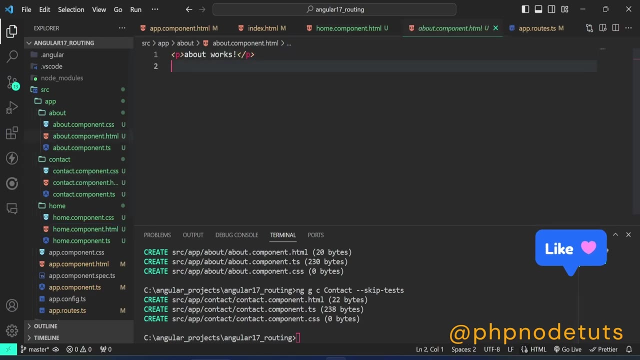 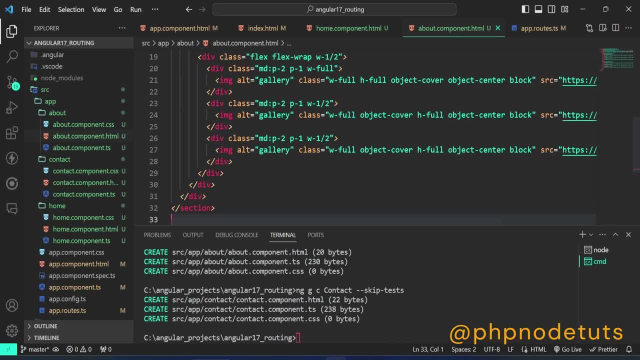 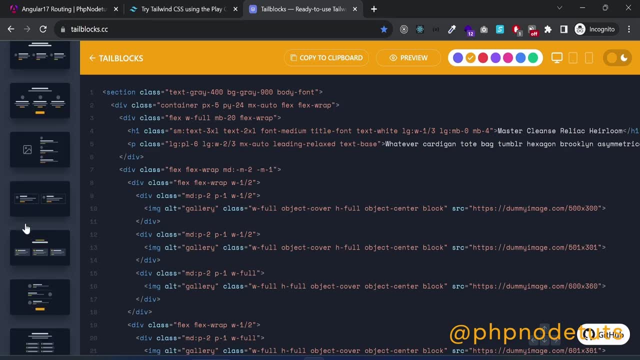 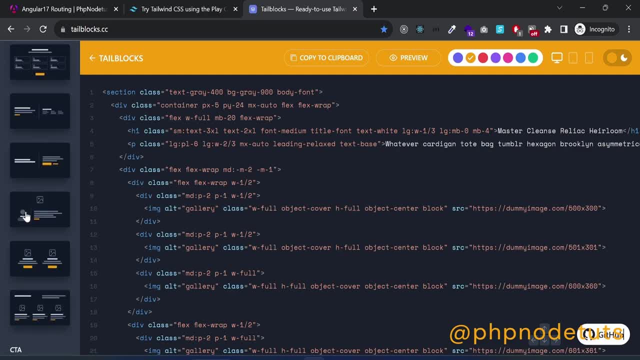 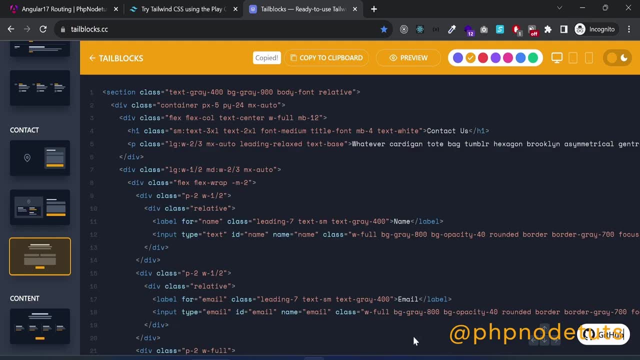 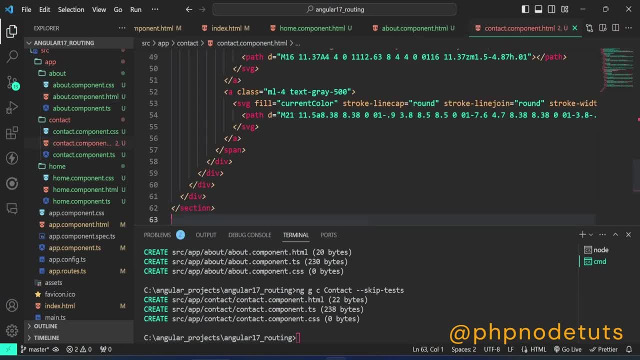 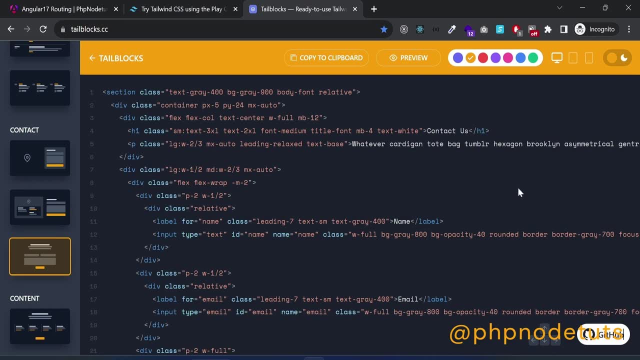 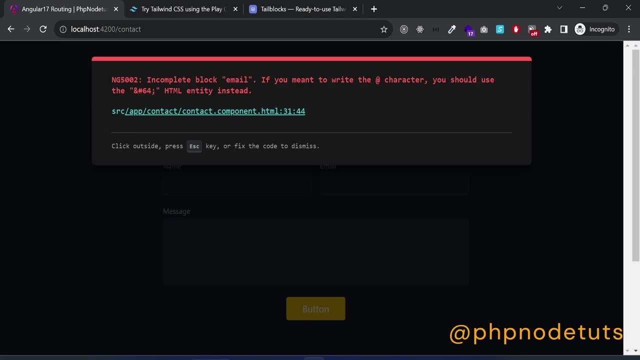 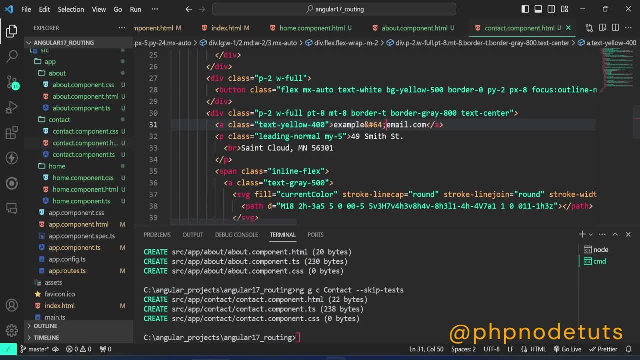 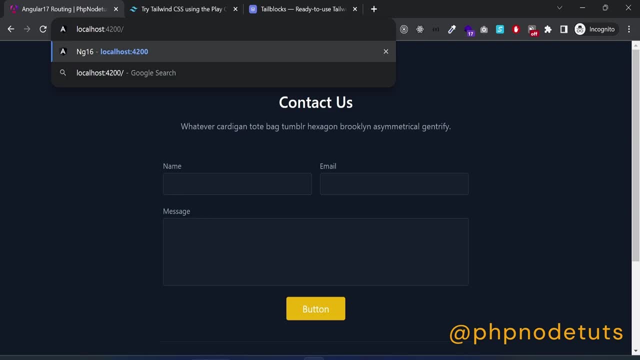 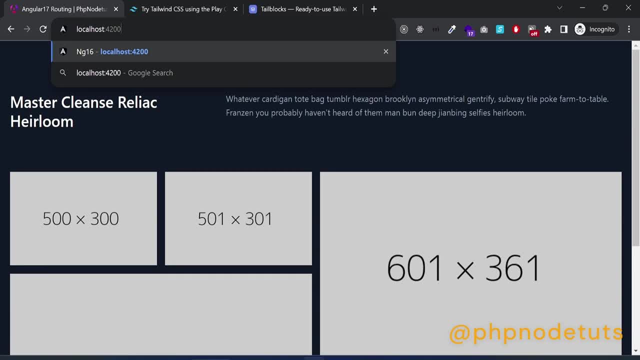 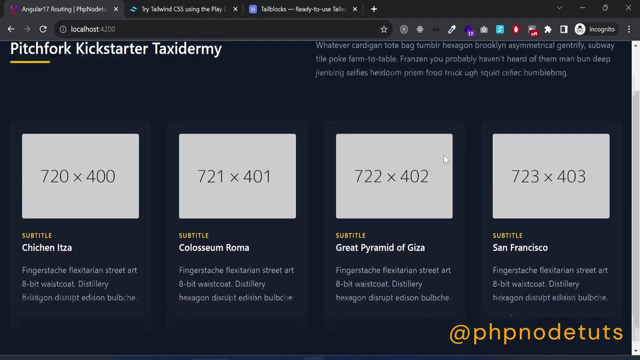 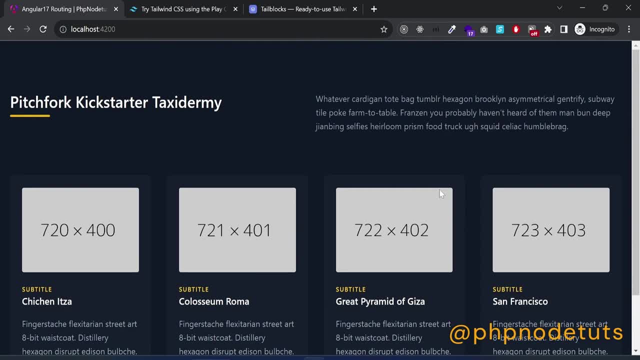 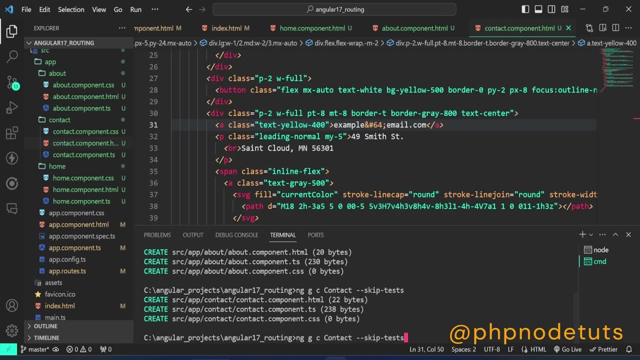 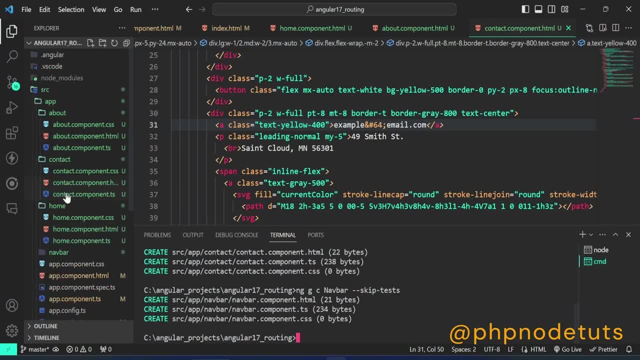 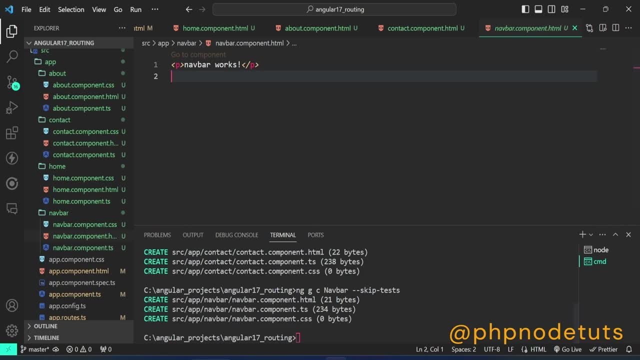 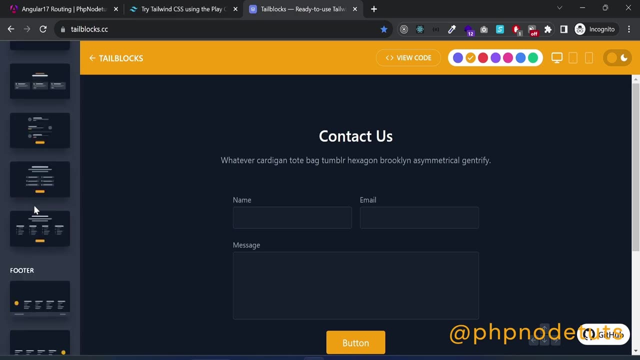 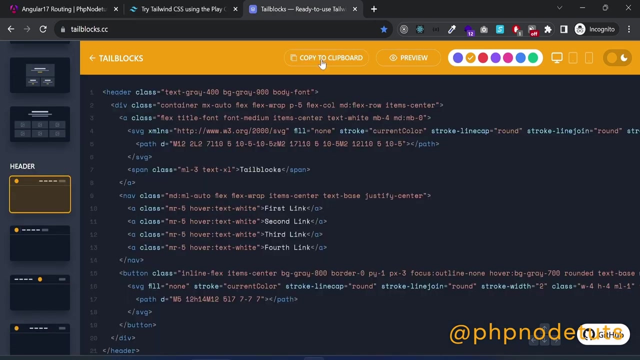 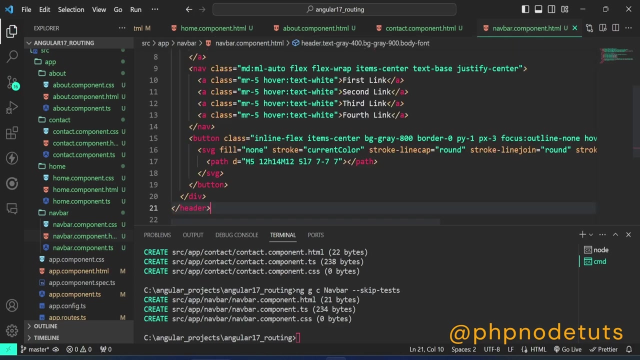 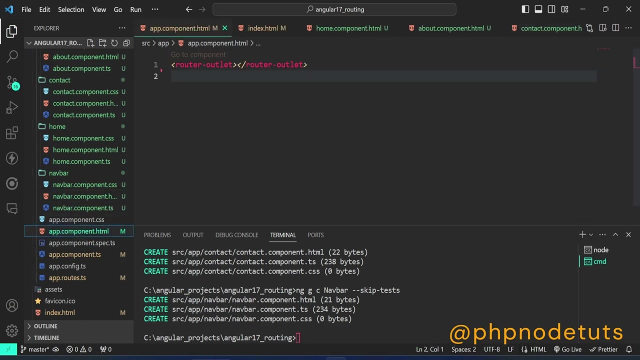 files inside app slash navbar folder. It will not create spects test file. Select this template block. Now click on view code and copy the code In navbarcomponenthtml file. remove the paragraph and paste the code. Now open appcomponenthtml file and add the app navbar selector. before router outlet: 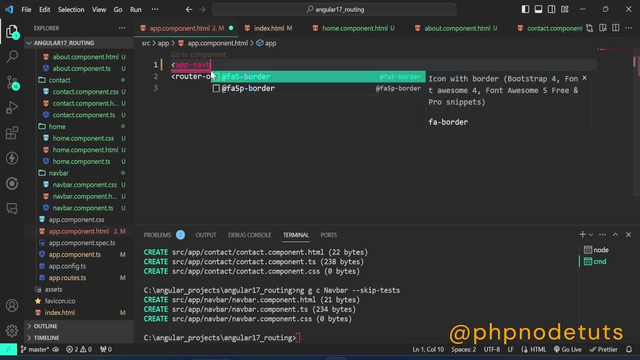 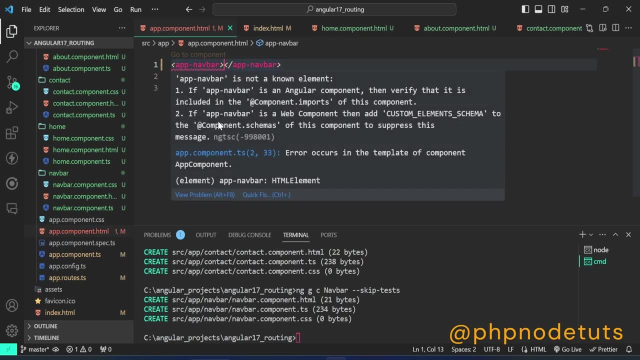 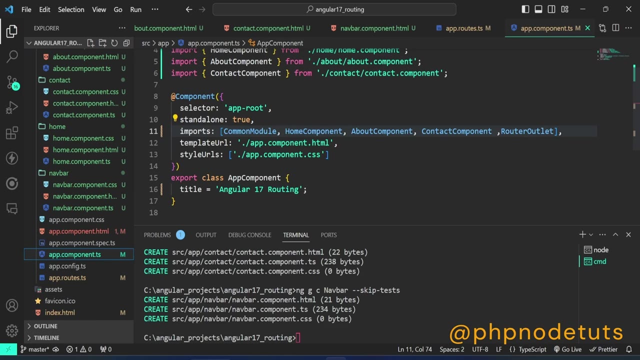 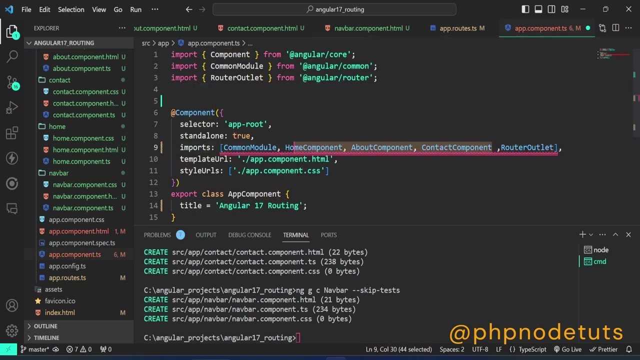 as we want to display the navbar on all pages, You can see the error. app navbar is not a known element. To fix this error, we need to import the navbar component in appcomponentts file. In appcomponentts file. remove the imported components: home component about component and contact component. Also remove these components. 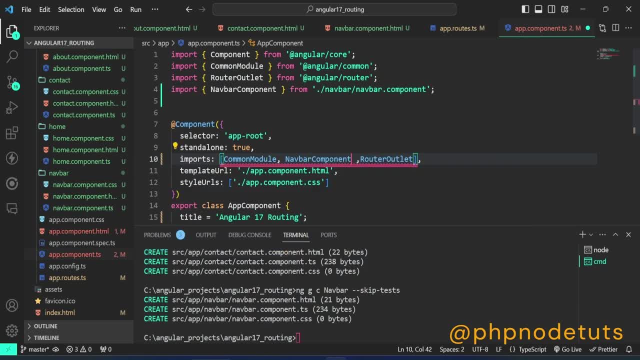 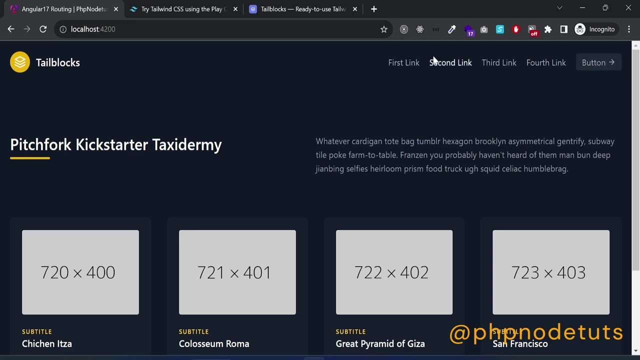 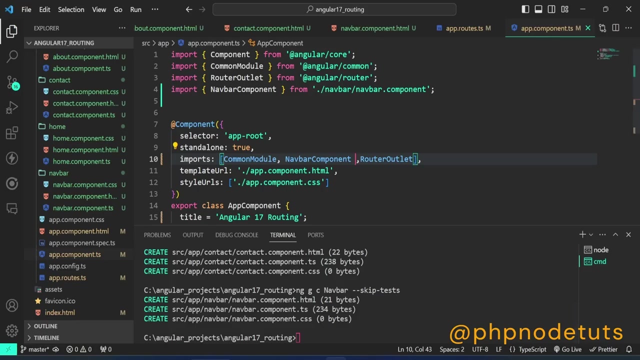 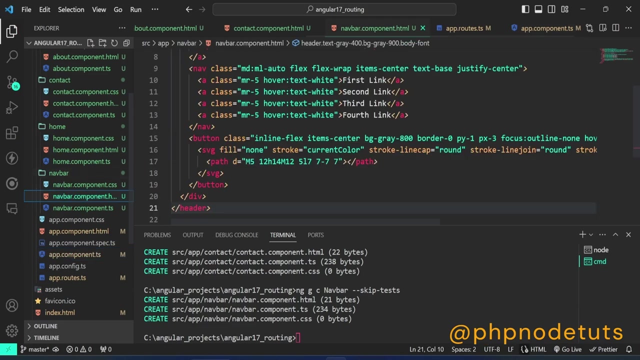 from the imports array Now. add navbar component in the imports array and import the component. Now. if you try to open the links, they will not open because we haven't added the router link directive to the navbar links. Open navbarcomponenthtml file. 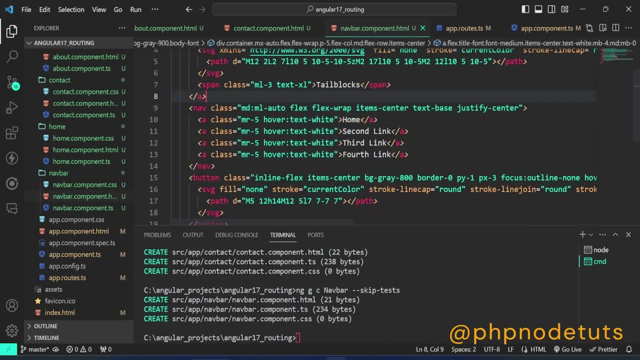 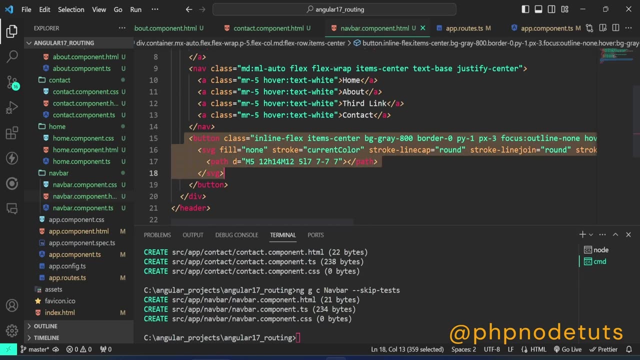 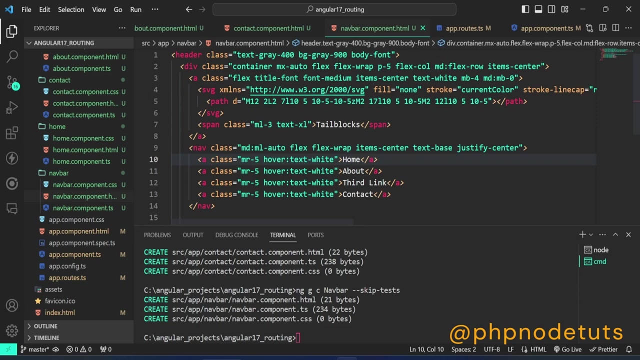 Remove the text and type home. In second link type: about Here. remove the text and type contact. Remove this code Now in the a tag of home link before the class type route In the a tag of about link type: router link equals in double quotes: slash about. 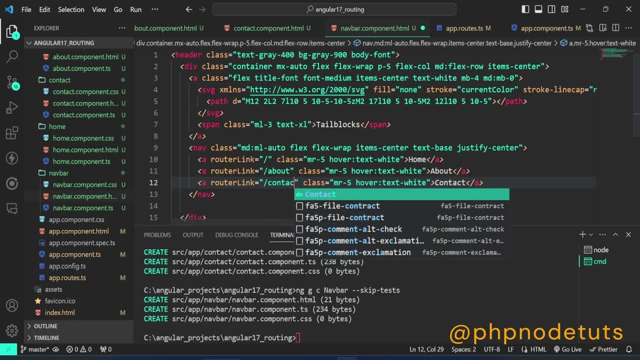 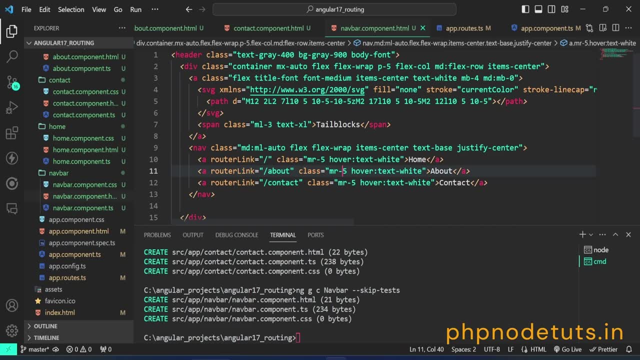 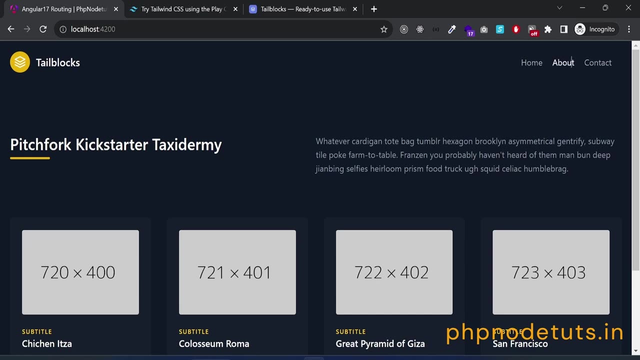 In the a tag of contact link. type: router link equals in double quotes slash contact. Now if you click on the links in the navbar, the pages will not open because we haven't imported the router link directive in the navbarcomponentts file. 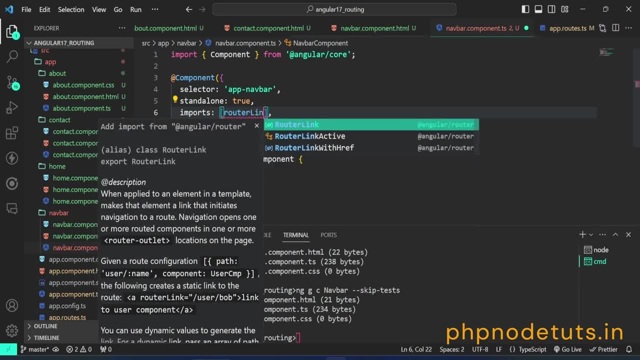 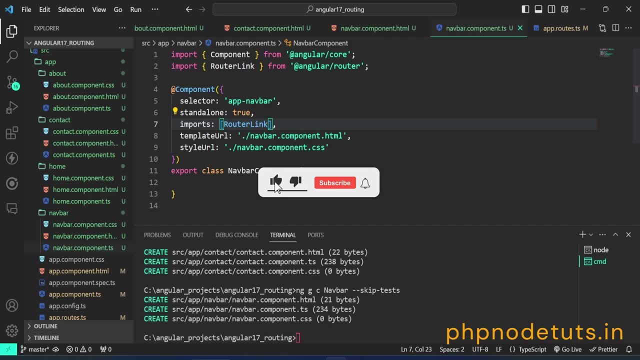 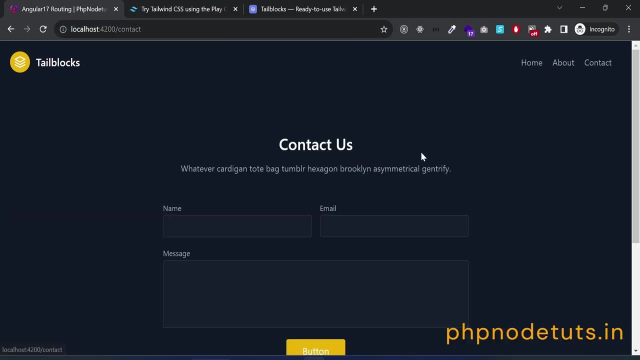 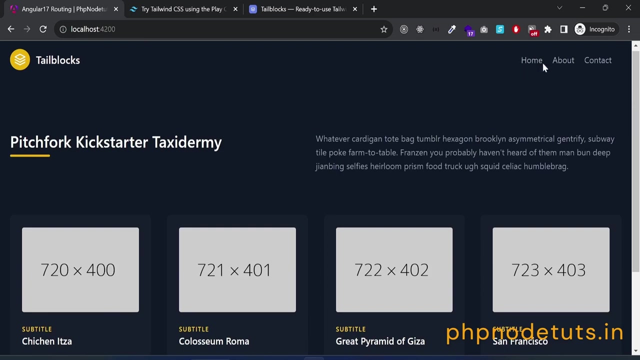 Open navbarcomponentts file. add router link directive in the imports array and import it. Now. if you click on the navbar links, all the pages will open Here. all the pages are opening, but we need to add an active link indicator so that when a particular 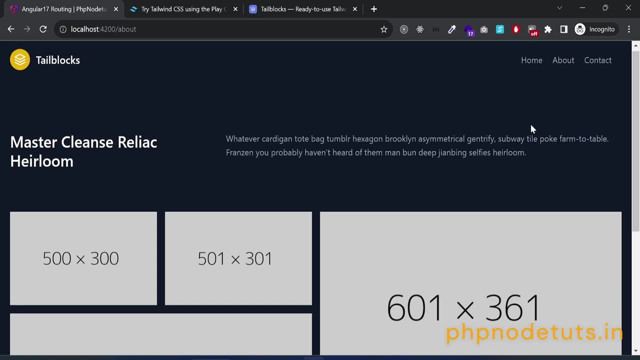 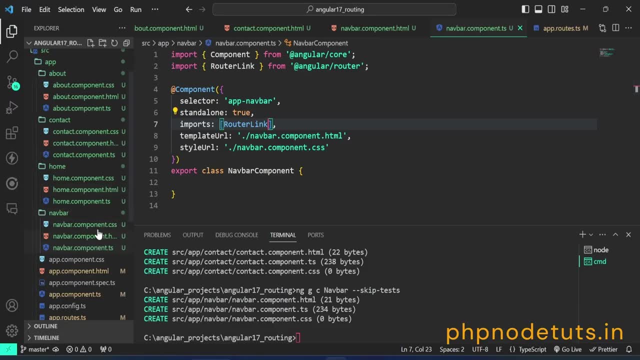 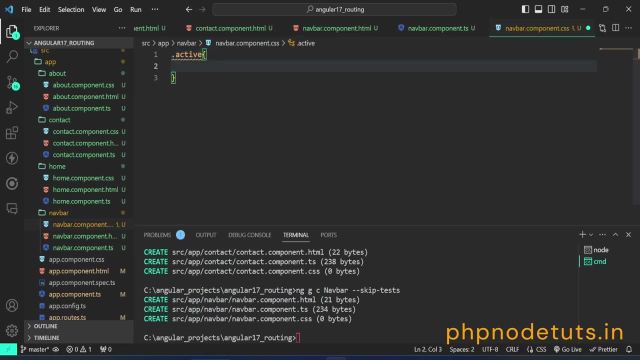 page is opened. the pages are not opened. Now, if you click on the navbar links, all the pages will open. opened, a border will be displayed under the corresponding link. Open navbarcomponentcss file and addactive class. Add border, transform and transition property and their values in the active class. 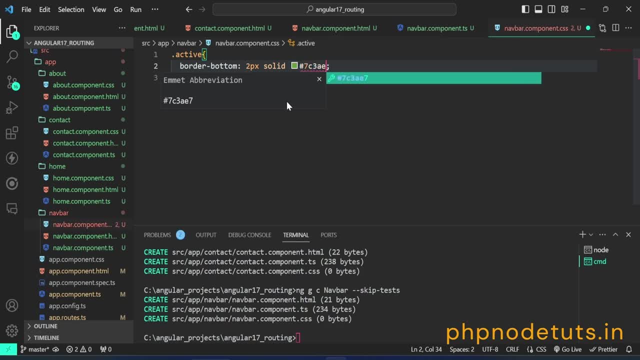 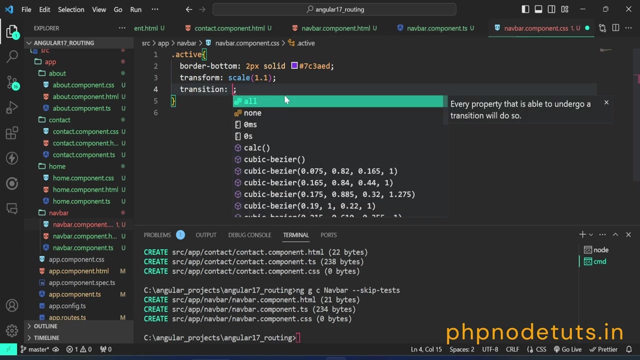 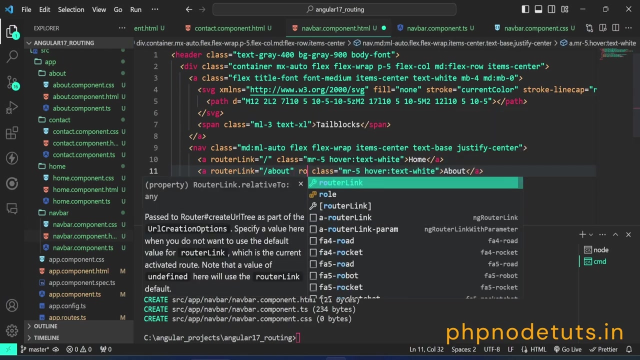 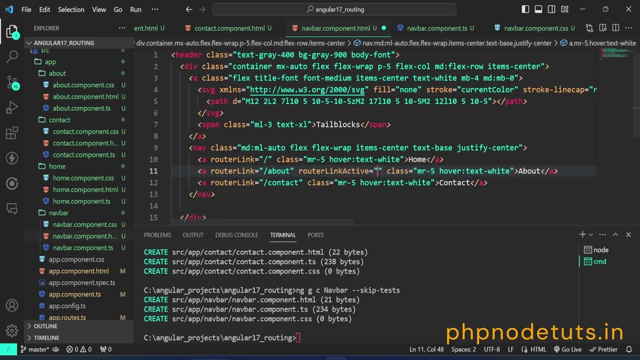 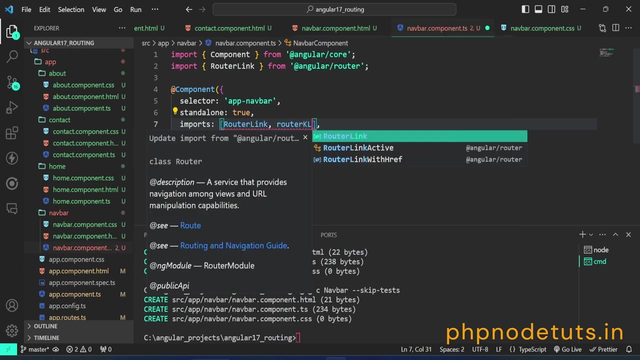 Thank you for watching. Thanks for watching Now. add router link active equals in double quotes active. where router link active is an angular directive and active is the active class. Copy this code and paste inside all the links: Open navbarcomponentts file. add router link active directive in the imports array and import it. 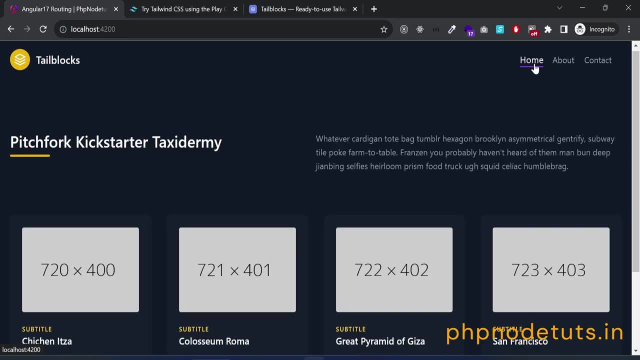 You can see that the active link is displaying under the link when we open a page. But there is a small issue. The active link is displaying under the link when we open a page. You can see that the active link is displaying under both the home and about or contact links. 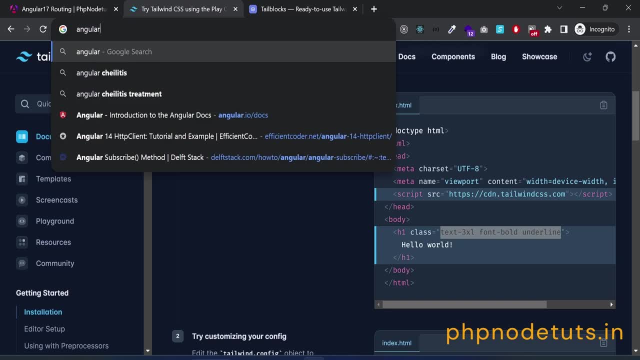 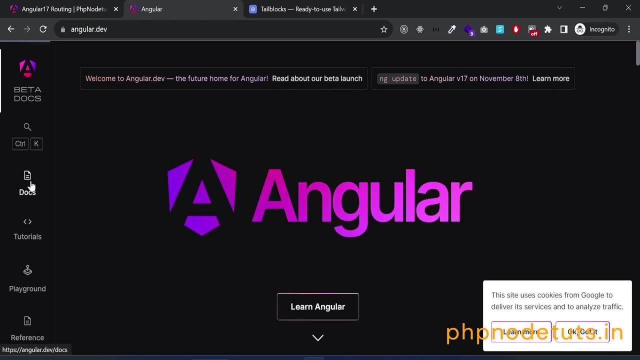 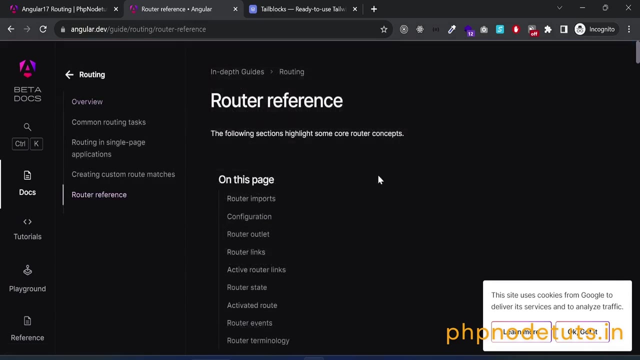 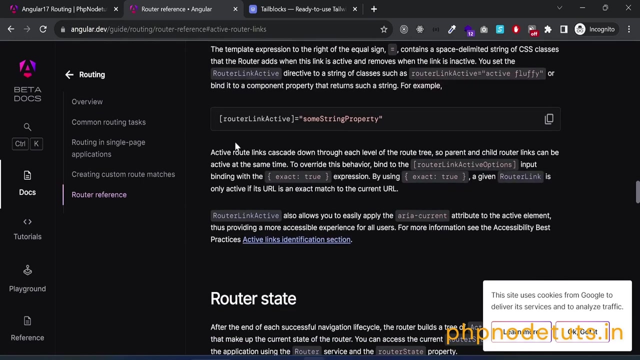 Open angulardev website, which is the new website for angular documentation. Click on the docs link Now. click on the routing link Now. open router reference. Click on active router links. Scroll down Here. you can see that active route links cascade down through each level of the route tree. 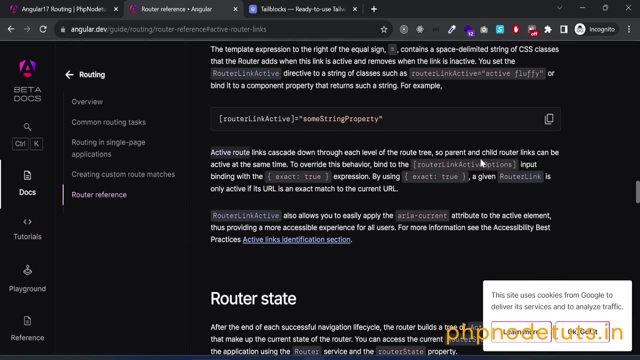 So parent and child router links can be active at the same time. To override this behavior, bind to the router link active options input. binding with the exact colon true expression. By using exact colon true, a given router link is only active if its URL is an exact match to the current URL. 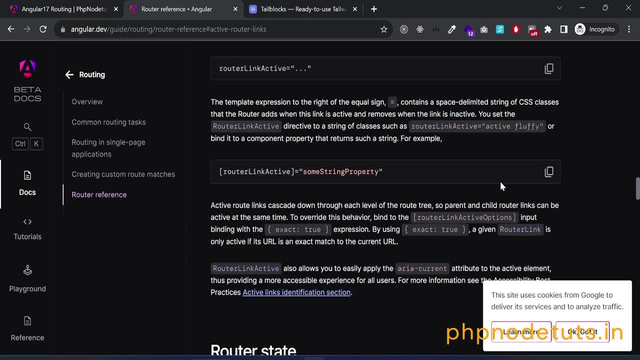 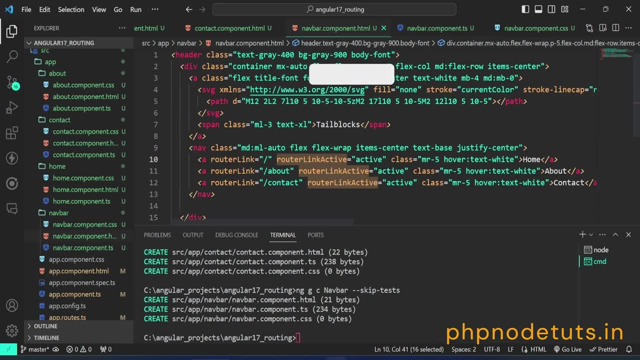 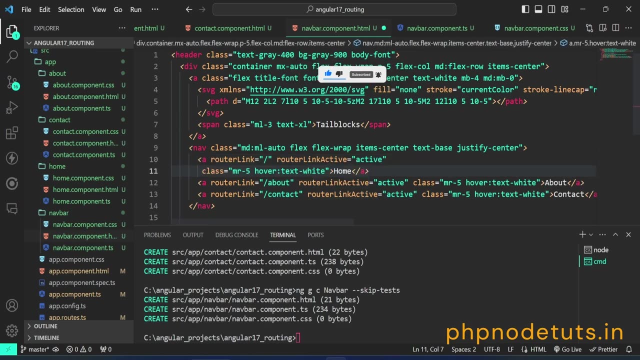 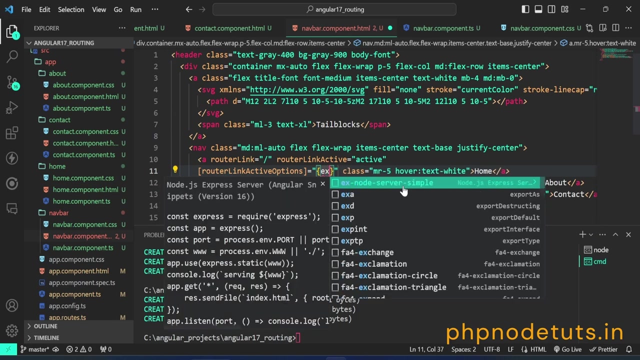 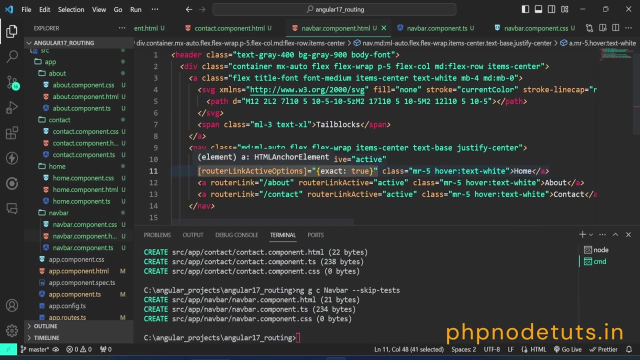 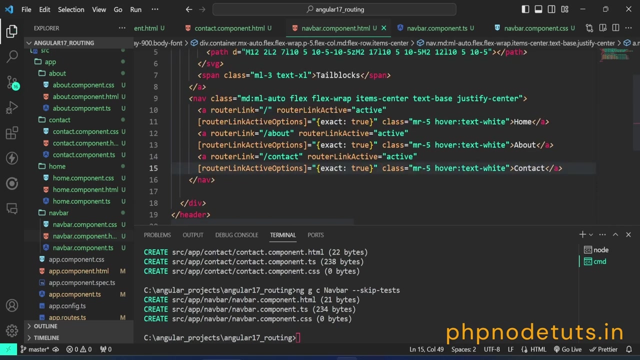 03 For 05 06 07 08: 20, 30, 31, 22, 32, 23, 24, 25, 26, 27, 28. the link active directive. Now, if you open any link, the active class border will only be displayed under the link. 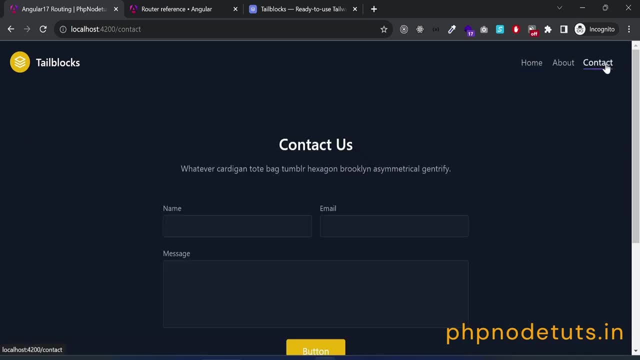 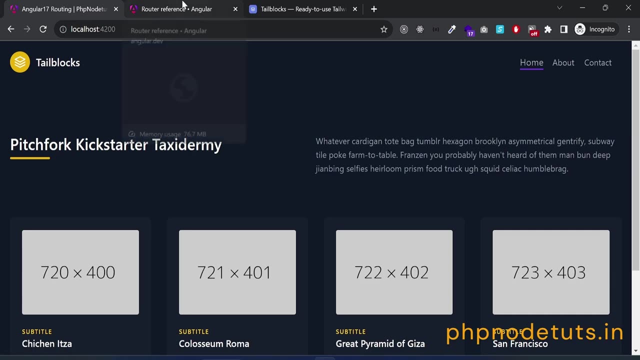 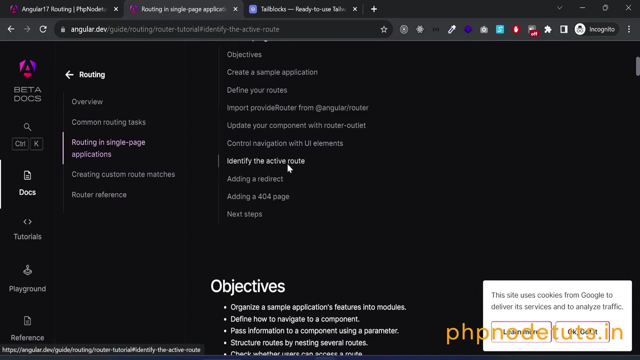 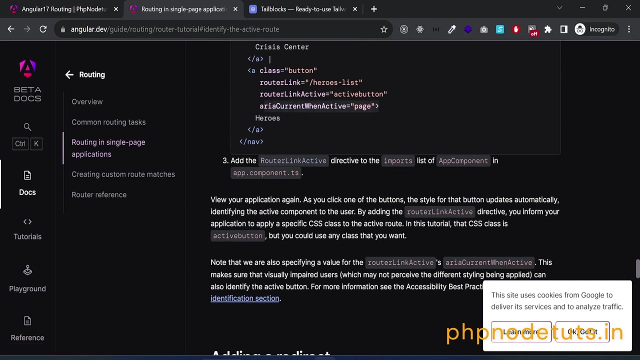 of the page that is currently open. Click on Routing in Single Page Applications link. Now click on Identify the active route. Here you can see: aria-current when active equals page. Aria-current when active is a input which sets the aria-current to a specified value. 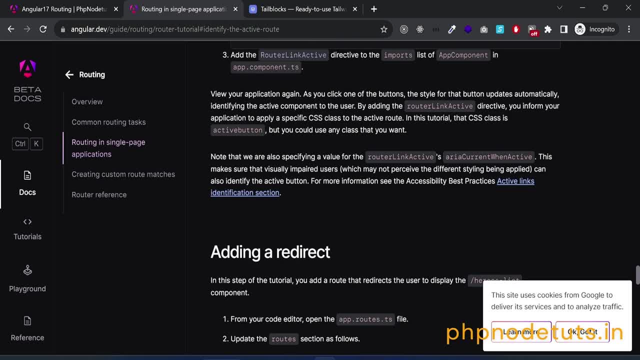 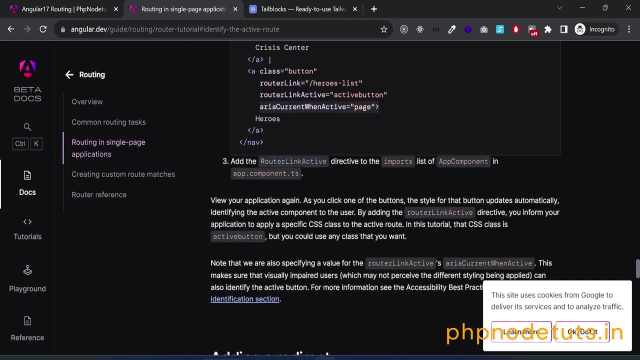 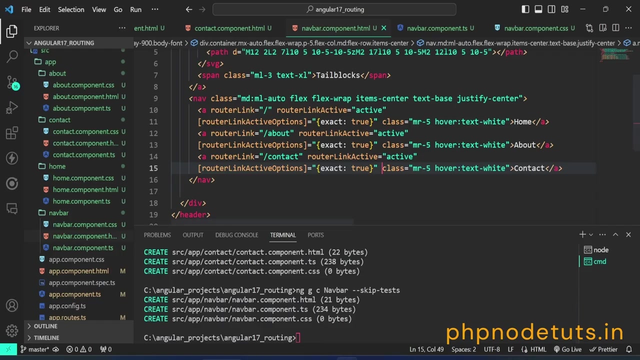 When the link becomes active. aria-current when active. makes sure that visually impaired users, which may not perceive the different styling being applied, can also identify the active button. Copy: aria-current when active- equals page. Add aria-current when active equals page to all the links after router link: active options. 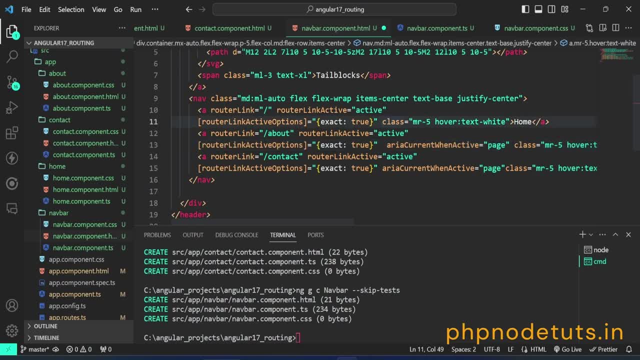 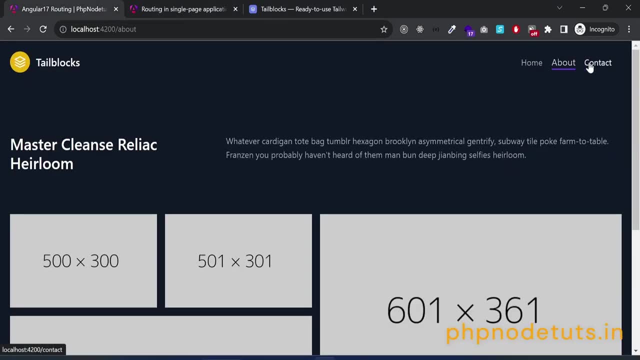 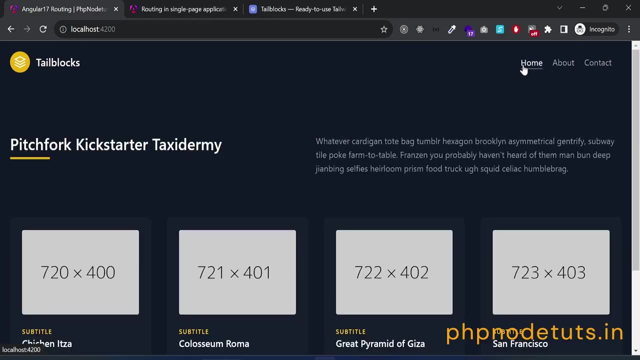 You can see that all the links are functioning correctly Here. you can see that we are on home page, but the title is not changing. If we go to the contact page, the same title is displaying. Now let's add a new link. 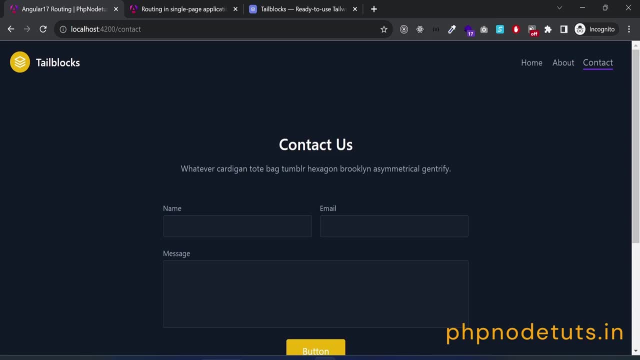 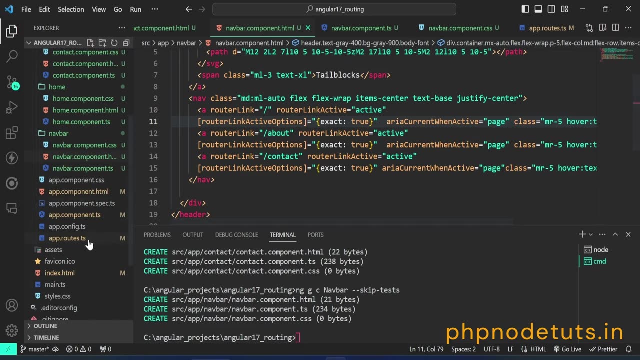 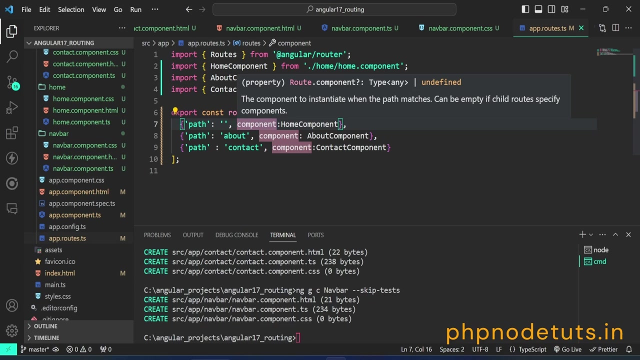 If we go to the contact page the same title is displaying. We can look at the page request page displaying Open approotts file. Here we will add the title property after the path in all the routes, In single quotes type- title, colon and in single quotes type the title of the page. 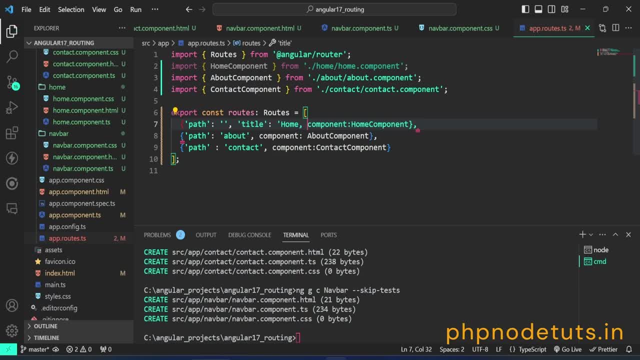 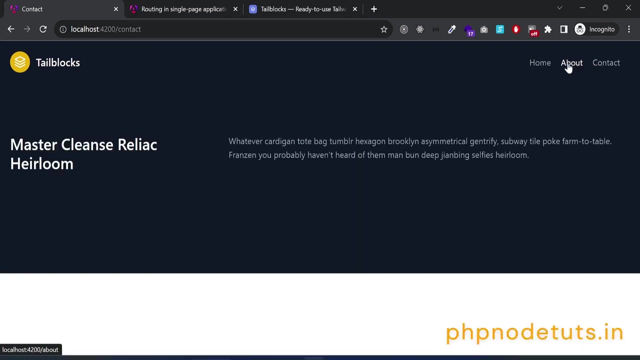 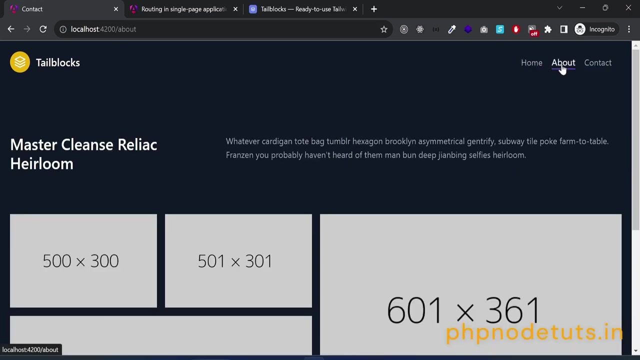 Add a title property and specify the title of each page in all the routes. Now you will see that when you go from one page to another, the title of the page changes. Now if a user types a route that doesn't exist, we need to display a 404 page- not found page. 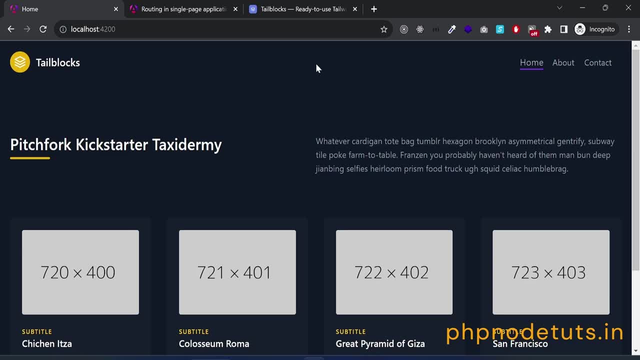 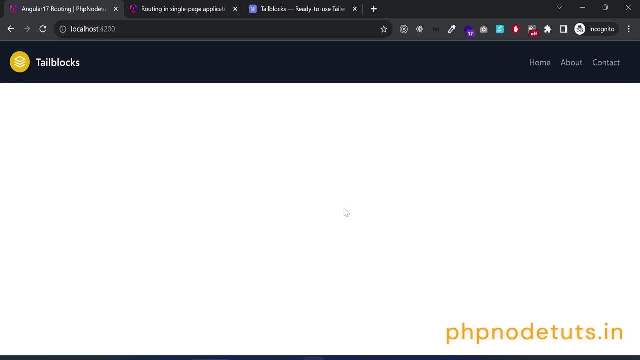 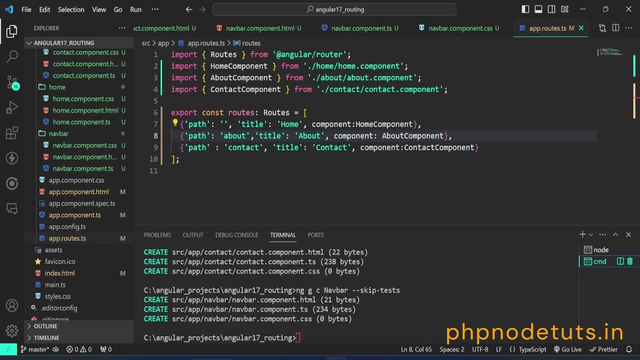 After localhost, colon 4200, type something randomly and you will see a blank page displayed with the navbar. Now let's create a page not found component. In your terminal, type the command ng, space g, space c, space page not found space. dash, dash, skip dash. 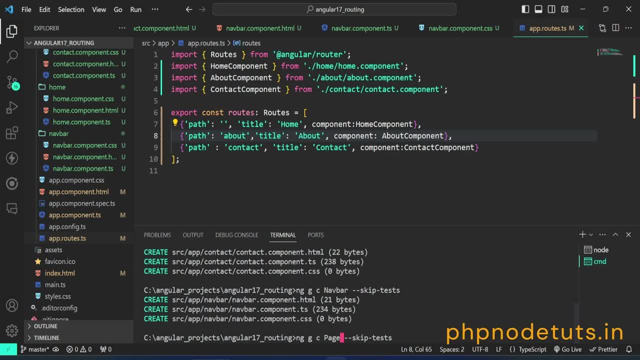 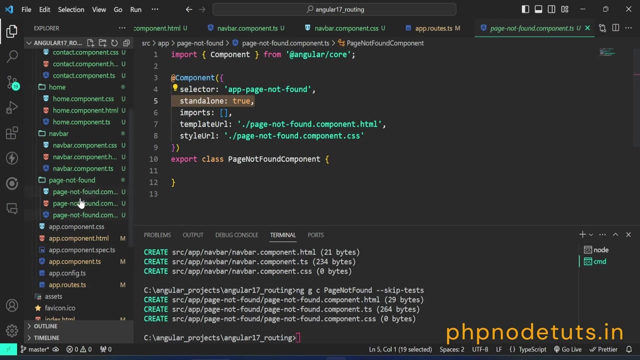 tests. This command will create page not foundcomponentcss, page not foundcomponenthtml and page not foundcomponentts files inside app slash. page not found folder. It will not create spects test file. Open page not foundcomponenthtml file and add this code: 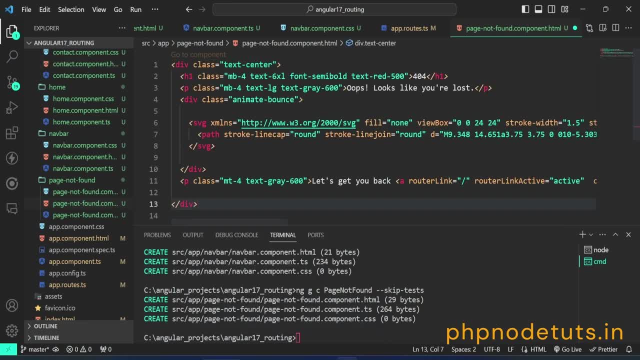 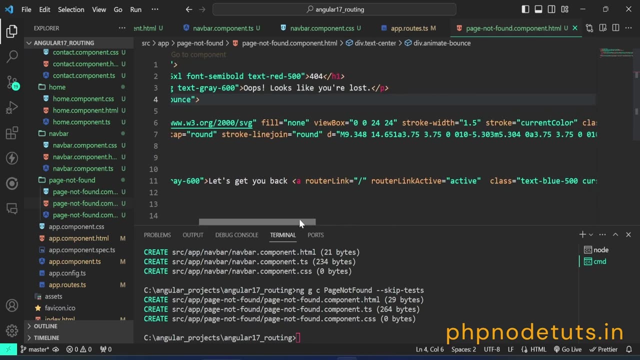 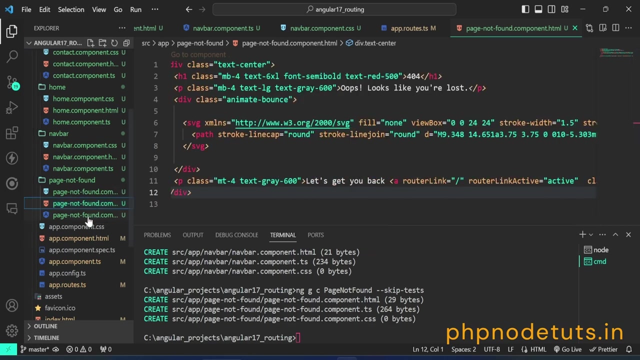 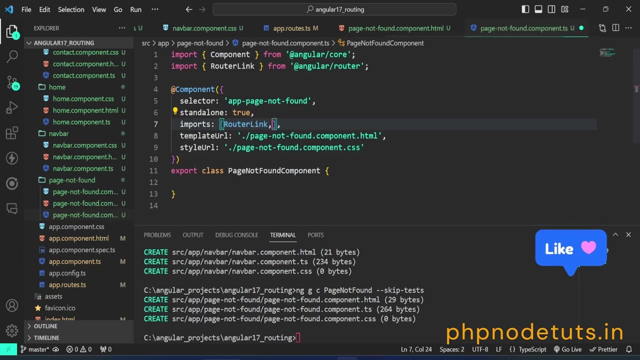 Which will display a 404 page- not found text- and a link to go back to home. Now open page not foundcomponentts file and add router link and router link active directives in the imports array. then import them. Click on routing in single page applications link. 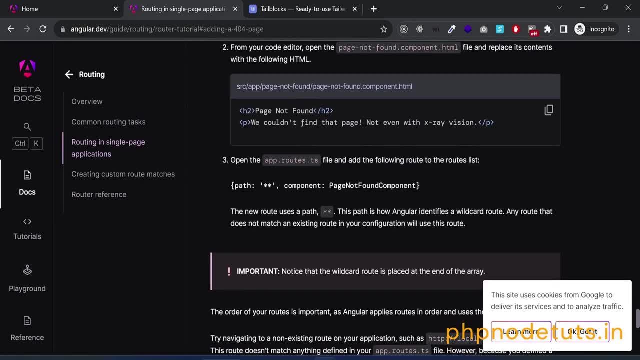 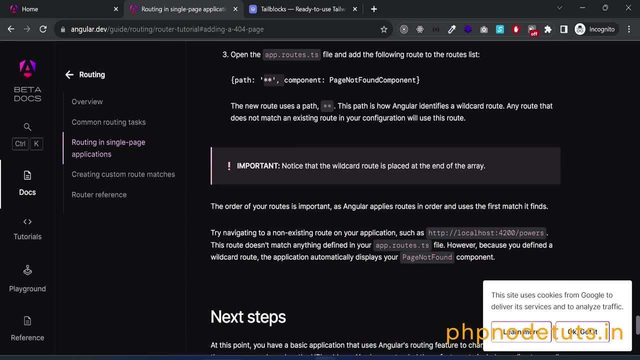 Now click on adding a 404 page. Here you can see that we need to add double star in single quotes in the path property. The new route uses a path double stars. This path is how Angular identifies a wildcard route. Any route that does not match an existing route in your configuration will use this route. 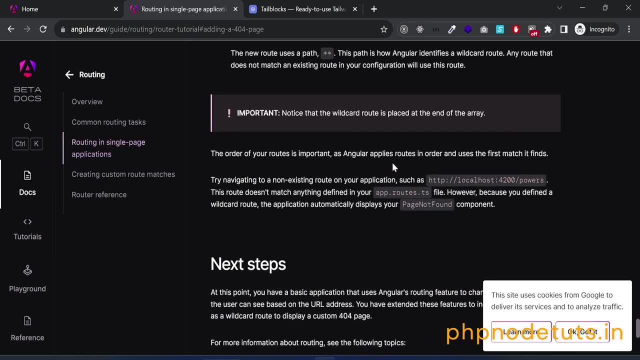 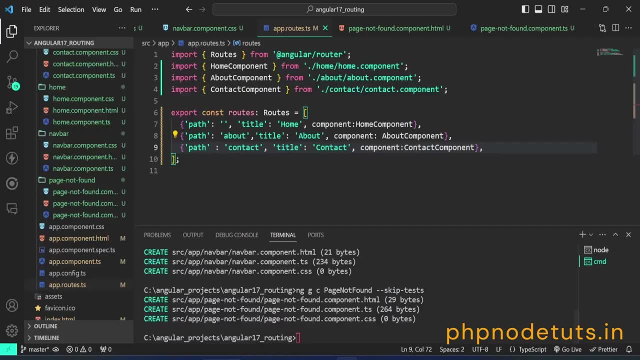 The wildcard route is placed at the end of the array. The order of your routes is important as Angular applies routes in order and uses the first match it finds. You can use this route for a random route. Now open approutests file and add the page not found route at the end of the array. 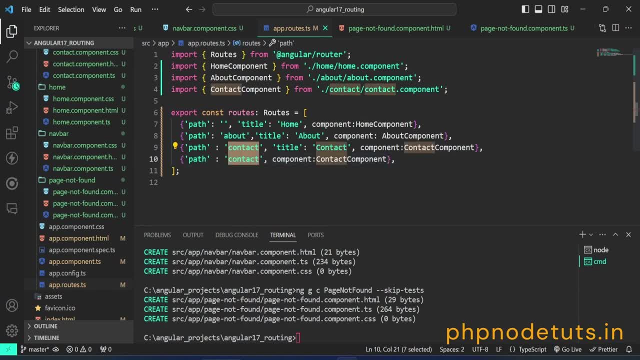 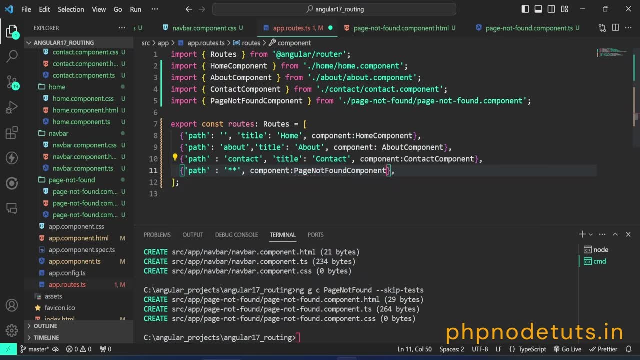 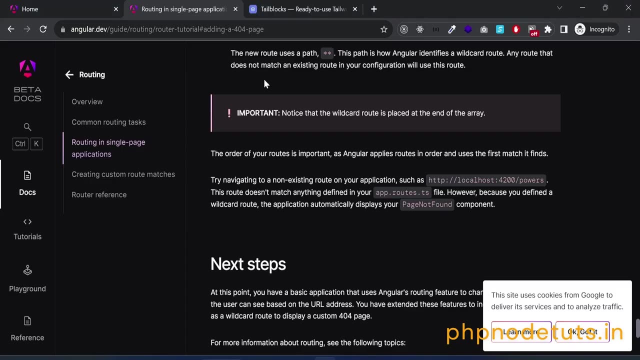 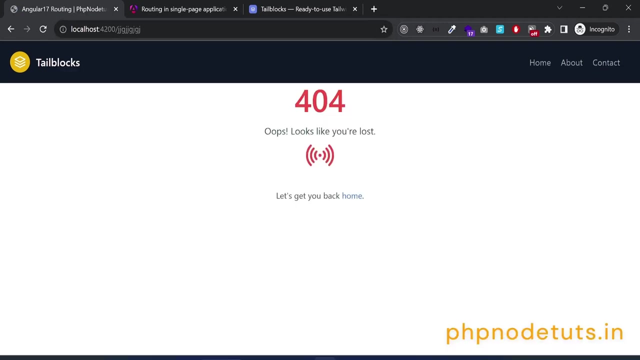 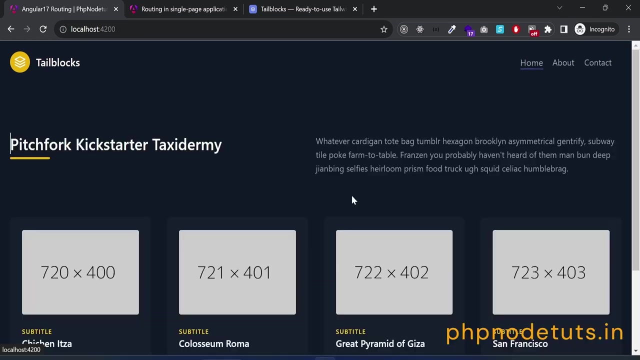 Do not forget to import the page not found component. Now, if you type a route that doesn't exist, a 404.pagenotfoundroute Or page not found page will be displayed. Click on the home link and you will go to the home page. 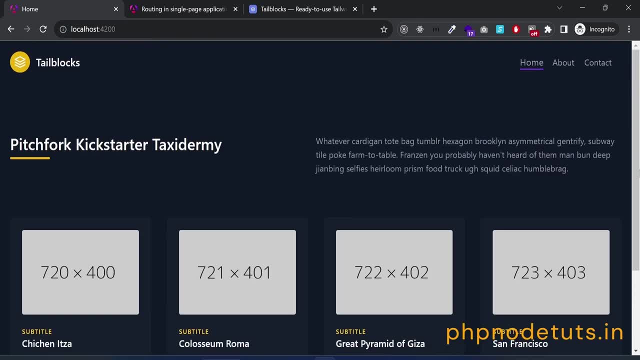 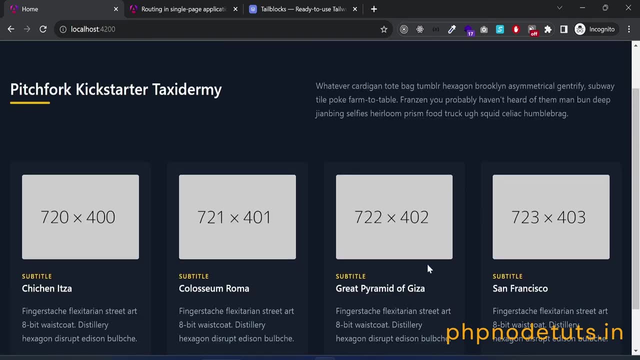 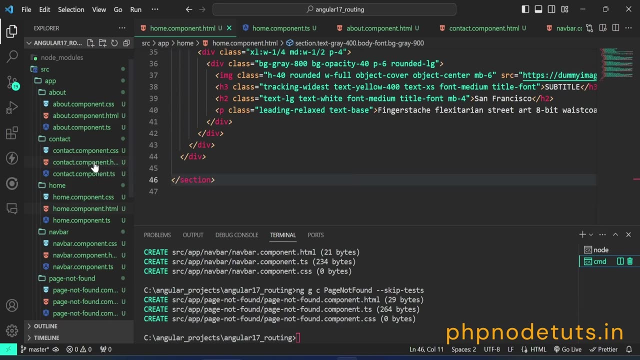 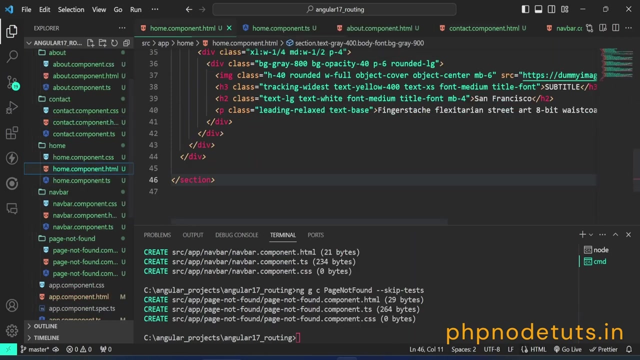 Now, let's say you have a link or button on the home page. When the user clicks on this button, they can go to another page. Open contactcomponenthtml file and copy this code Now. open homecomponenthtml file and paste the code before the closing section tag. 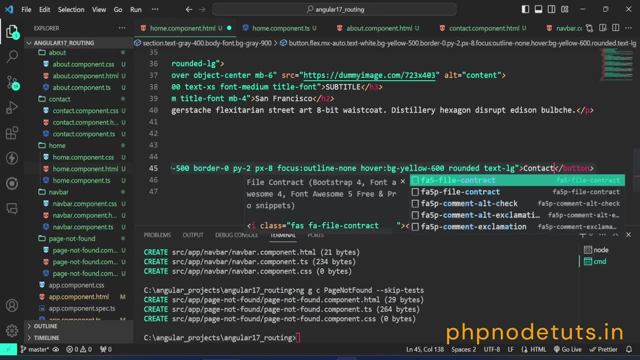 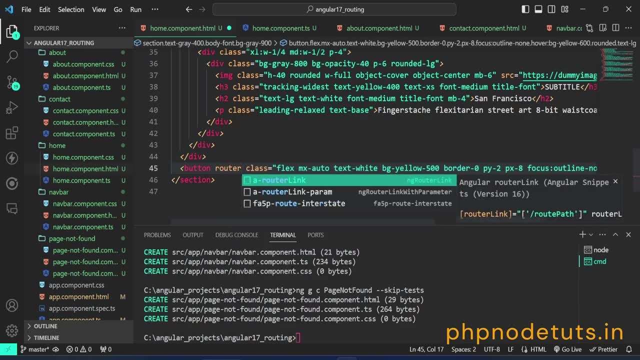 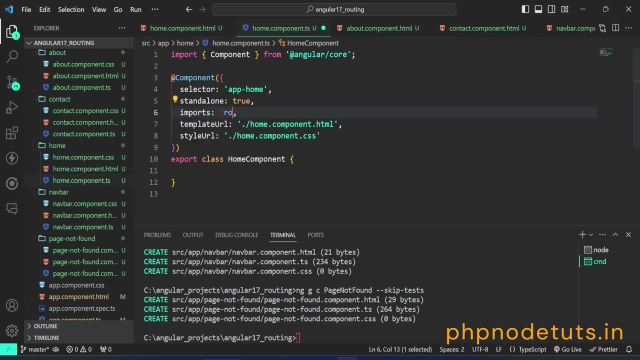 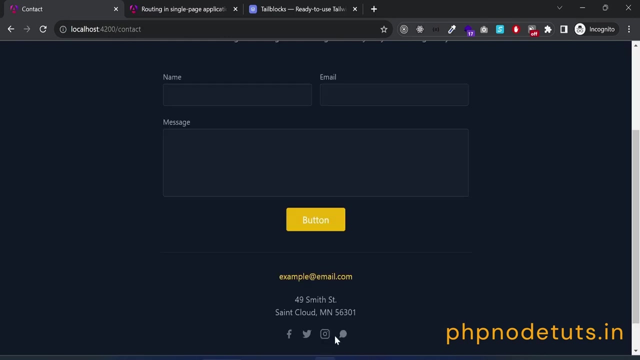 Replace the button text with contact Now. add router link equal. slash contact in double quotes. Open homecomponentts file. add router link directive in the imports array and import it Now. open home page and click on the contact button and you will go to the contact page. 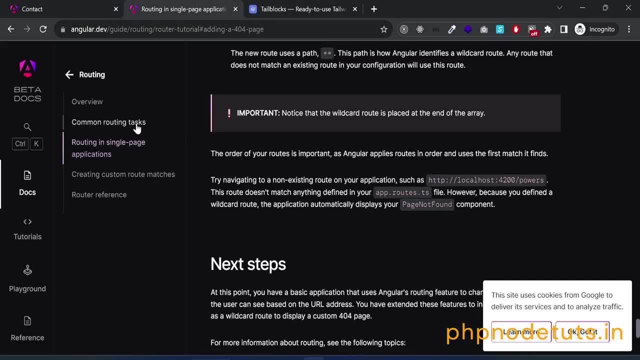 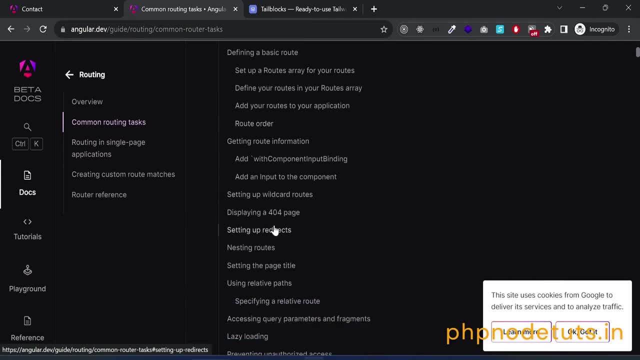 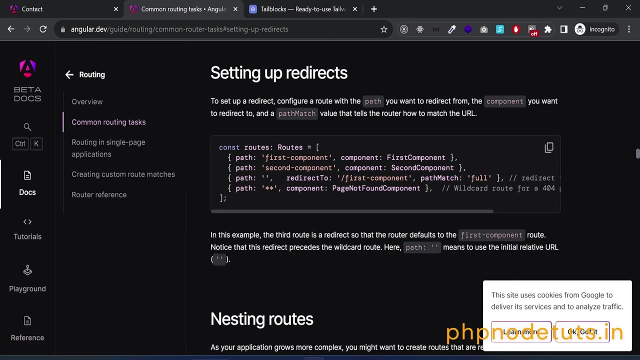 Now let's proceed to implement the redirect. Click on common routing tasks. Now click on. You can see that to set up a redirect, configure a route with the path you want to redirect from the component you want to redirect to and a path match value that tells the router how to match the URL. 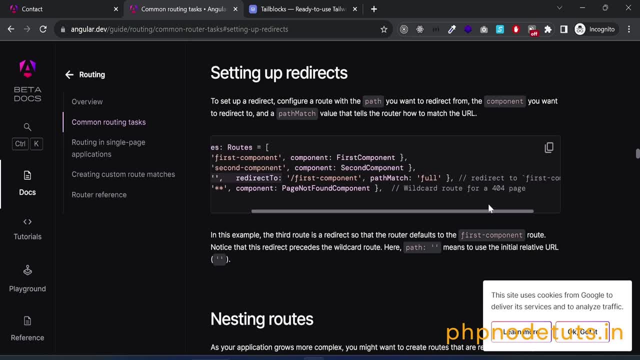 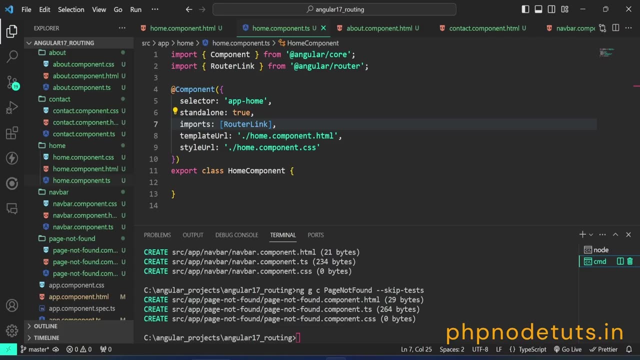 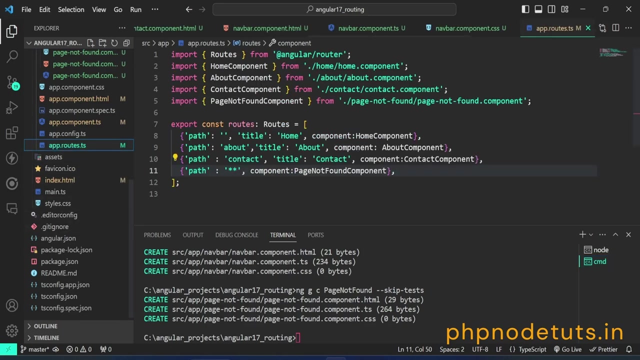 We need to add the redirect before the page not found route. Here the third route is a redirect so that the router doesn't have to add a new route. Notice that this redirect precedes the wildcard route. Now open approutests file. 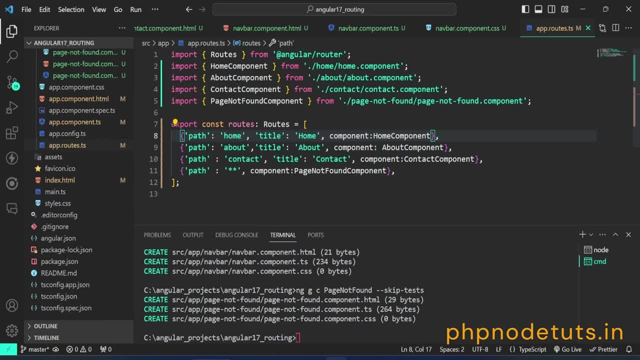 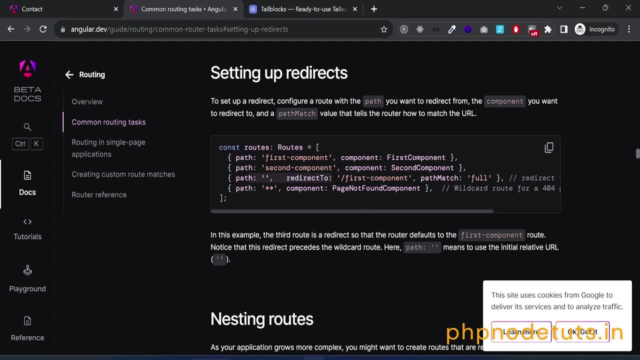 In the home route, add home in single quotes to the path property. Now, after the contact route, add a route that redirects the user to display the home component. These details will be passing this route to your user. Now, if a user in our Android service, sua aшая email, probably won't understand, portiku and request it. 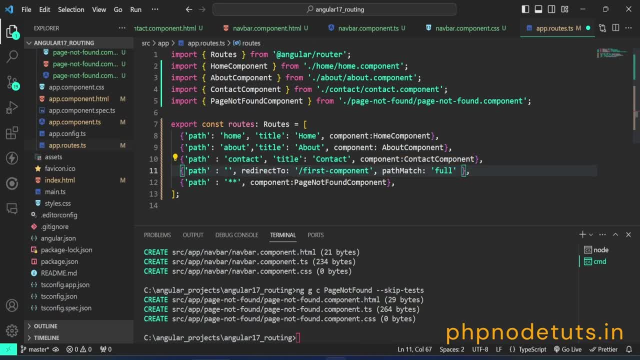 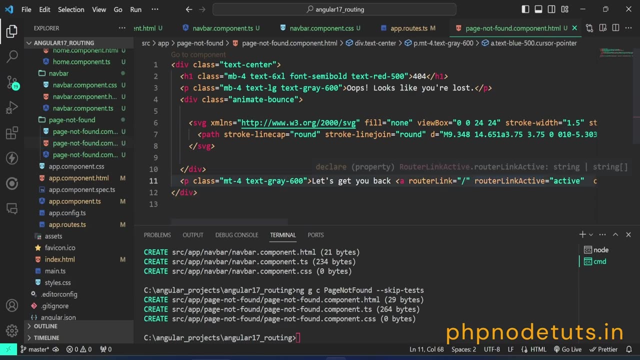 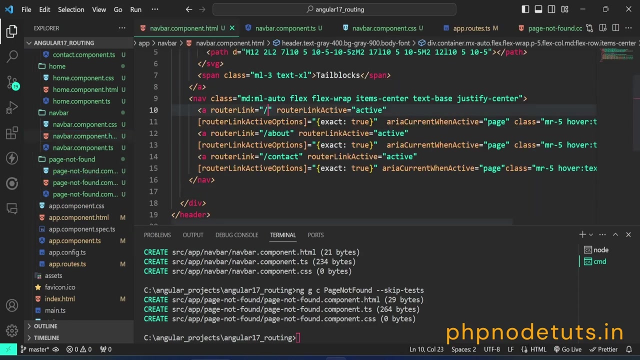 Let's change portiku to her TBO. Copy this code. Paste the code here. Replace first component with home. Open page notfoundcomponenthtml file Type- slash- home in the router link. Open navbarcomponenthtml file Type: slash- home in the router link.